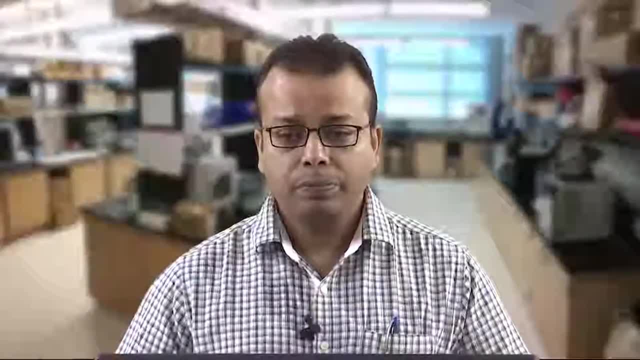 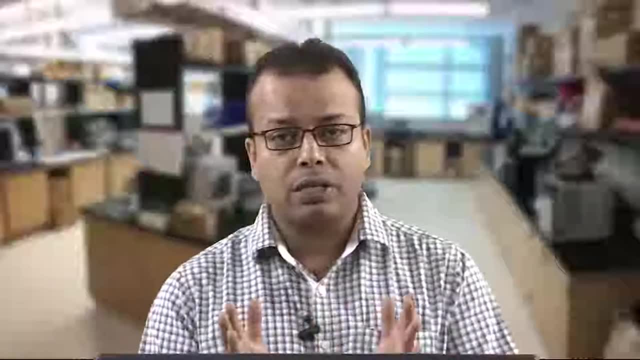 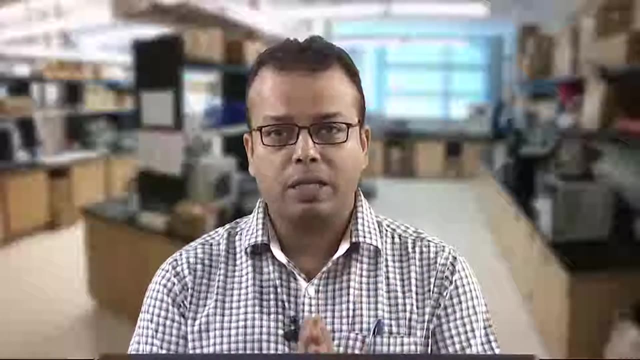 maybe the chemical properties or maybe the structural properties. So basically, actually this chapter is divided into so many subparts. So first we will discuss about the crystal structure, atomic bonding, then we are going to discuss about the different types of materials, like the metals, ceramics, polymers, some kind of advanced materials. 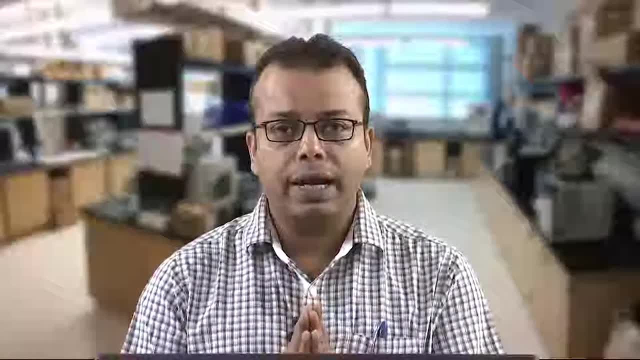 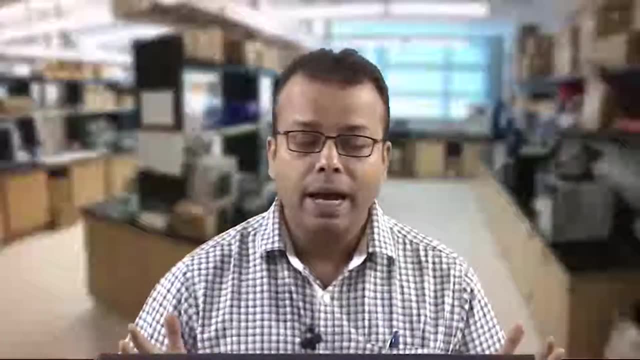 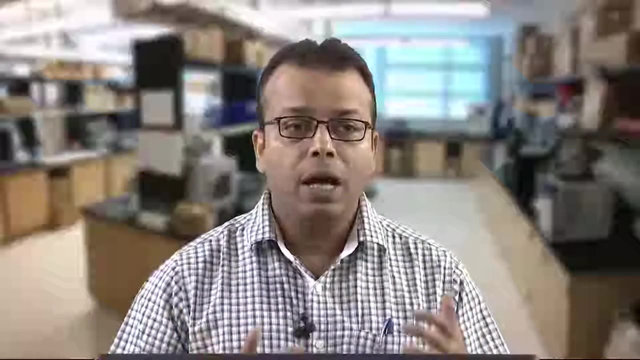 preparations and then later we are going to discuss that about the XRD generalization Generally, by which we can get the information about the crystal structure of that particular materials, and the last also, we are going to give some kind of new techniques like the XPS or maybe some kind of other methods by which we can get the crystal structure for. 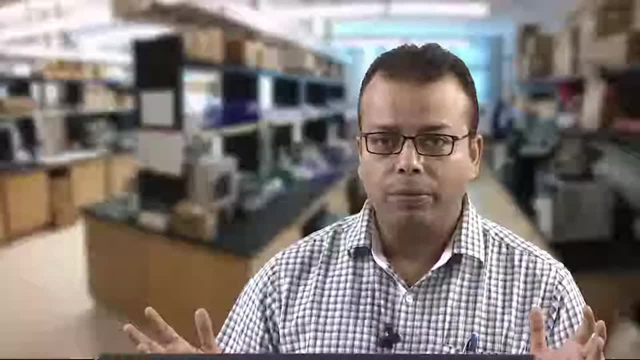 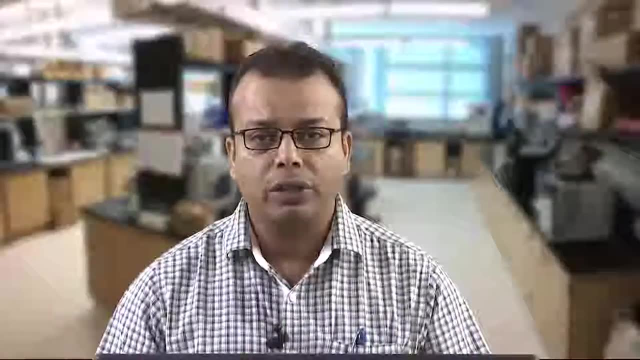 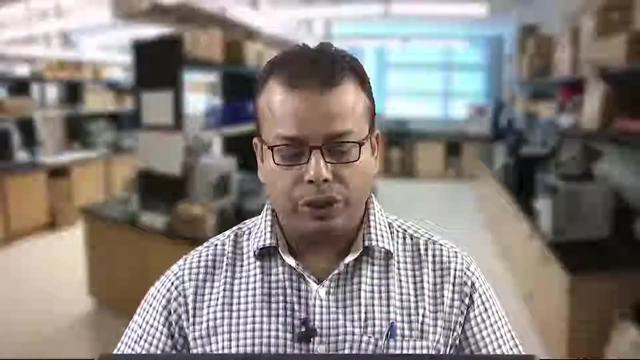 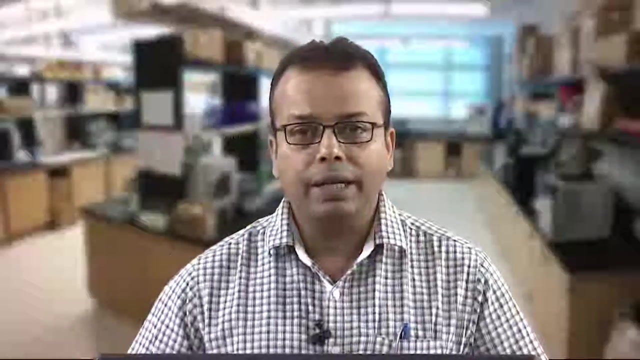 that particular material. So simple, in a single word, I can say that this subject will give a wide information about the crystal structure and their properties for a particular material. So today, actually, we are going to start our first lecture, which is nothing, the introduction lecture. So fundamental concepts of atomic structure and their inter-atomic bonding. 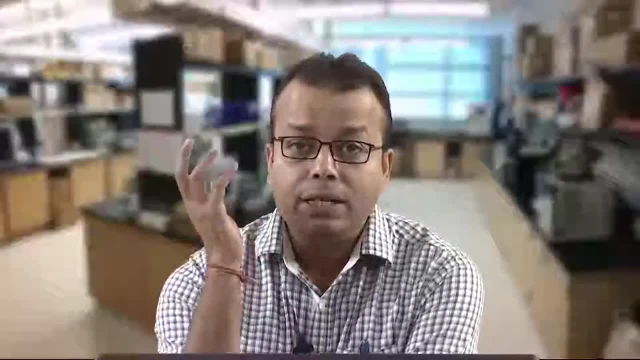 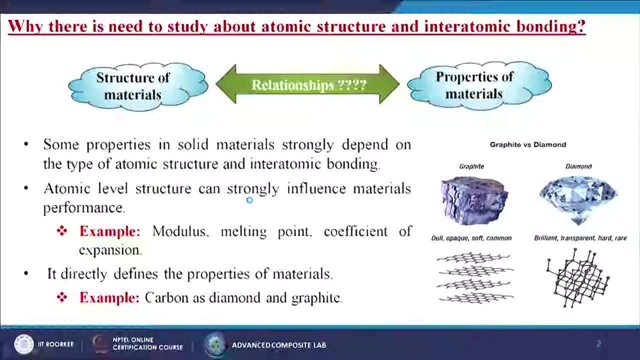 So first, before going to start, let us know that, why it is required to study the atomic structure and the inter-atomic bonding. So generally, in the structure of materials generally, what is the relationships when we are getting the properties of materials? So first is the 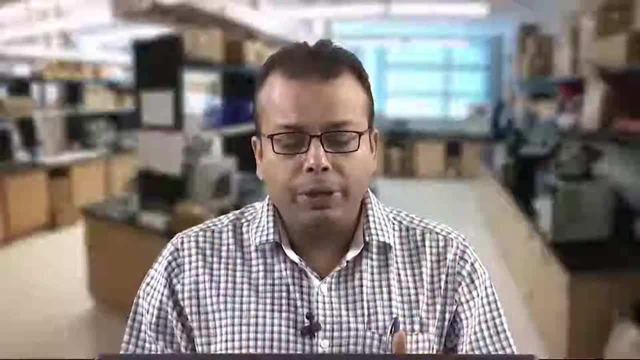 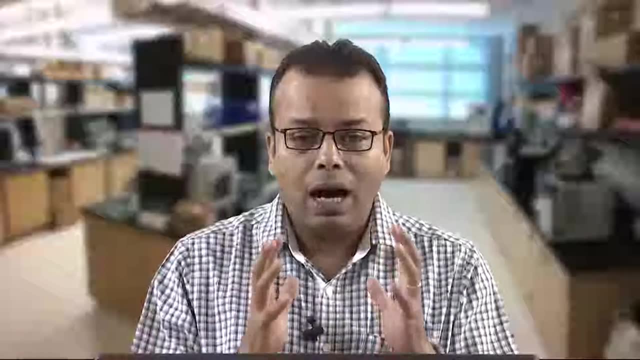 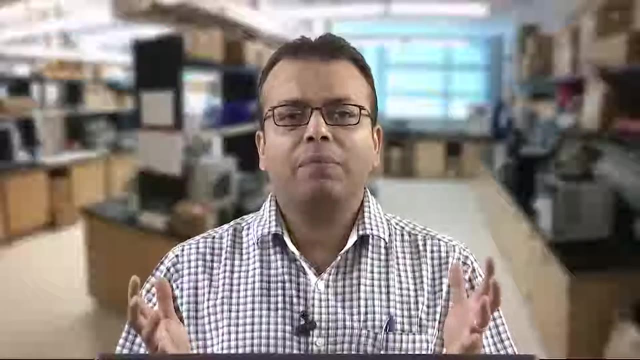 structure of materials And the properties of materials and in between the relationship. So relationship will give you the particular essence that how the material will behave, or maybe what kind of material I can add. So what will be the new crystal structure? formations means it is a some kind 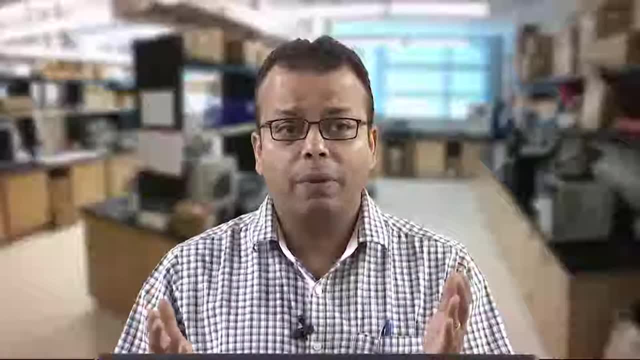 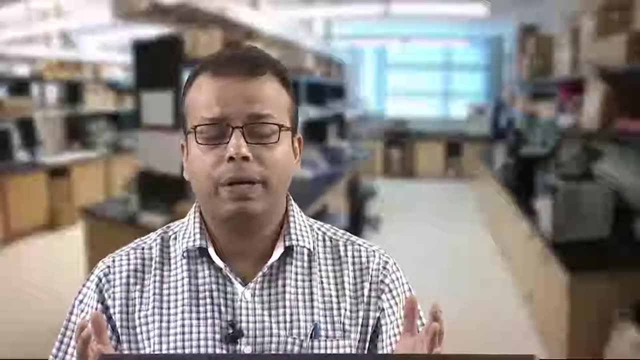 of in a single word. you can say that that is a some kind of X-ray kind of view of that particular material. from that we can get the information about the physical properties of that particular materials Or maybe about the chemical properties of that particular materials. So some properties. 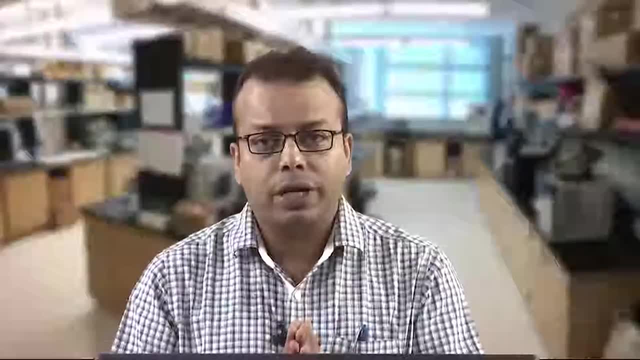 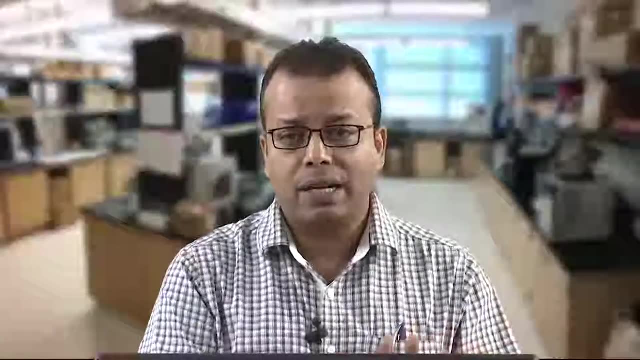 in solids strongly depends on the type of atomic structure and the inter-atomic bonding. This is well known fact. This we have gone to our in class 10 standards or maybe class 2F standards. So of course every material is having some atomic structure and the inter-atomic 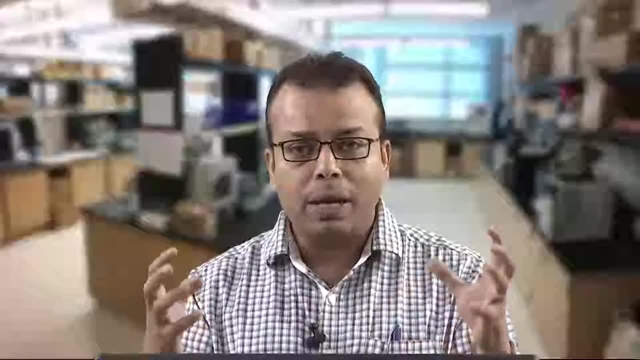 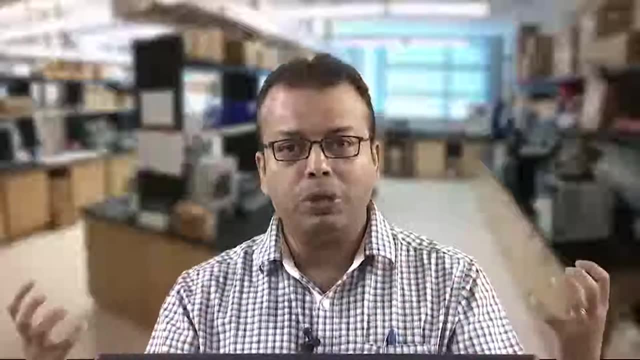 bonding, because the atoms are closely packed with some bonding, otherwise the atom can go randomly anywhere. So there should be some kind of inter-atomic bonding, So the atoms are closely packed with some bonding, otherwise the atom can go randomly anywhere. So there should be some force which can acts in between the atoms, So atomic level structure can strongly. 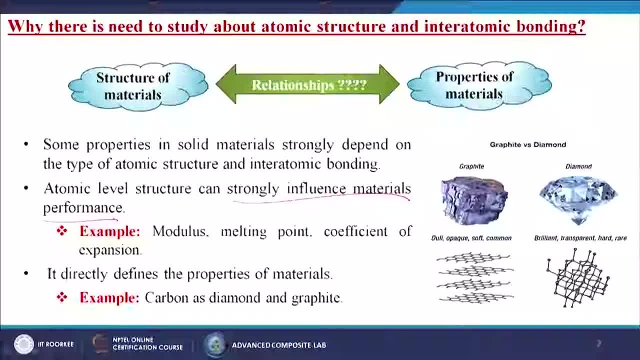 influence the material performance. So this is the vital point over there. So what are the material performance Generally? we can talk about the modulus, we can talk about the melting point, we can talk about the coefficient of the expansion. So it directly defines the properties of materials. Yes, of course, from that particular point of view. 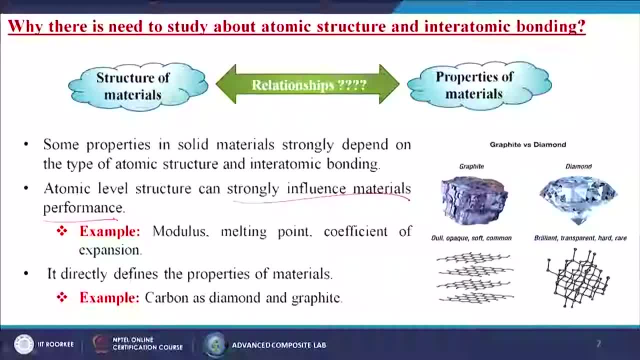 we can get the information about the materials: Carbon as diamond and the graphite. Here right hand side you can see some kind of things that graphite and diamond we have given the example. So graphite its looks like dull, opaque, soft, and the common materials means easily available When we are talking about 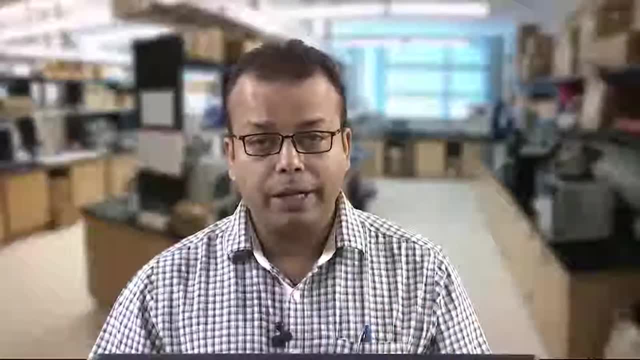 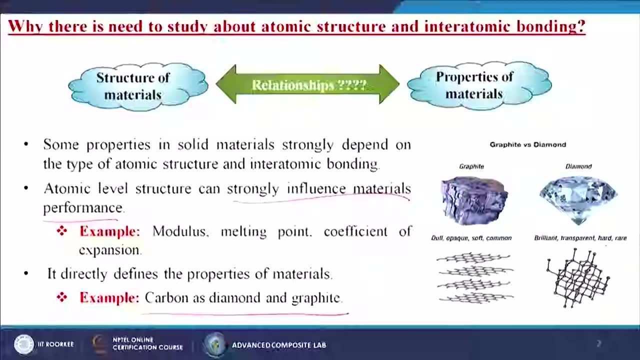 the diamond. it is very, very brilliant and transparent and it is having some glittering or maybe some kind of reflective in nature. It is very hard and it is also the rare earth materials, because it is not easily available. you can prepare it some kind of artificial. 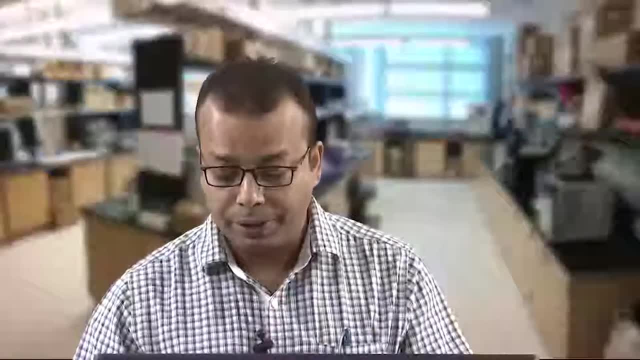 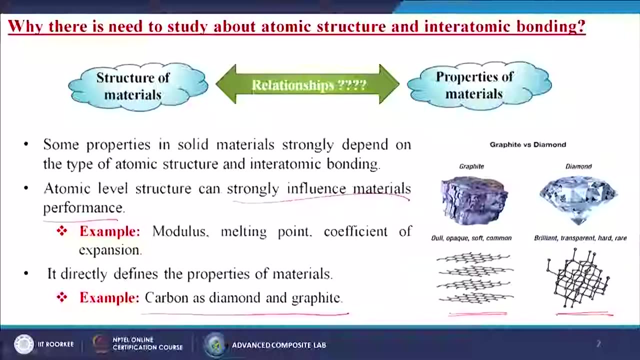 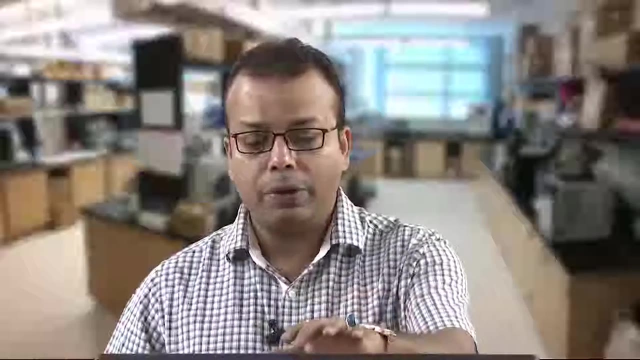 diamond, but with some help of high end equipment. So generally you can see the crystal structure of the graphite and you can see the crystal structure of the diamond also. this crystal structure of the graphite is the layer by layer stacking, and in the diamond it is a closed packed of the carbon atoms. 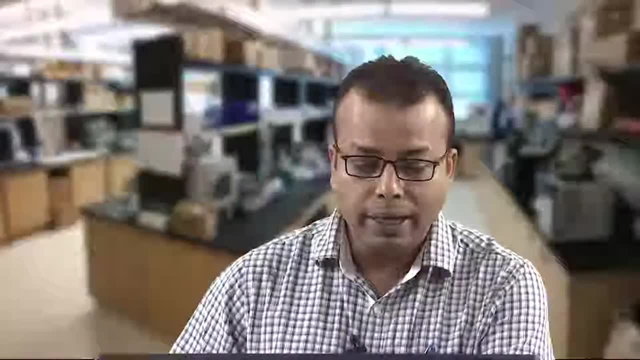 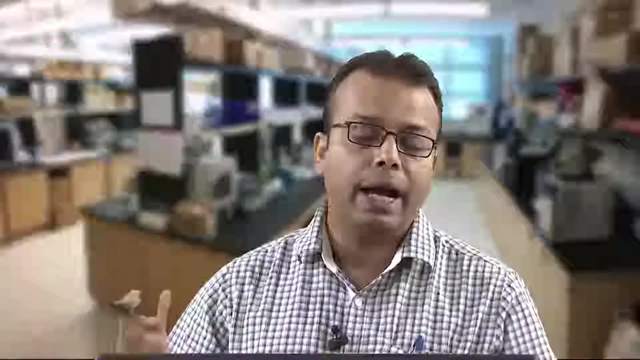 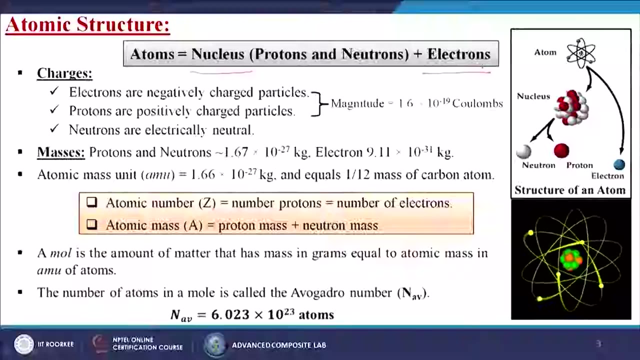 So first let us know what is the atomic structure. so generally, atoms is equal to nucleus. nucleus is constitute by two things, that is the protons and the neutrons, and another one is called the electrons. so atom is divided into two groups: one is nucleus, another one is electrons. 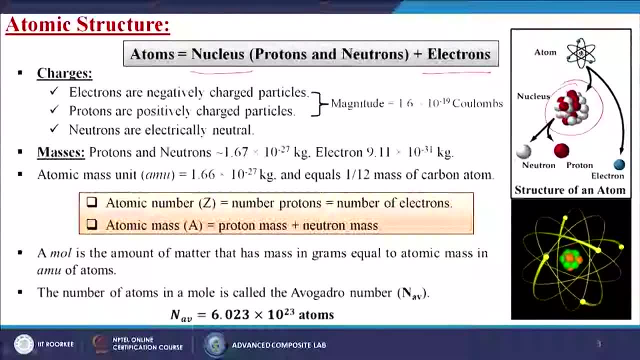 so here in this atom. so it is the nucleus of that material. so it is divided into two parts: neutron and proton, which is nothing but the nucleus, and another one is coming from electron. so charges, electrons are negatively charged, particles, protons are positively. 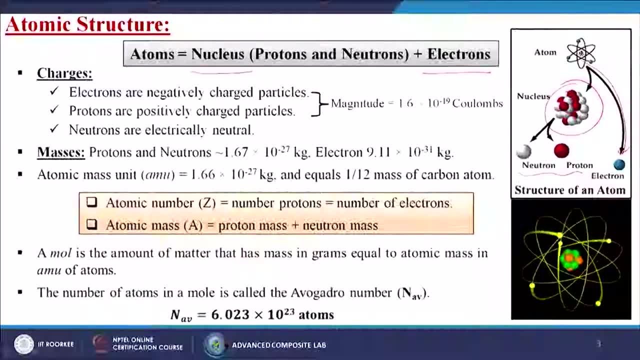 charged particles And neutrons are electrically neutrons. so this is the three characteristics of these three. so what is the magnitude of electrons and protons? Generally, 1.6 into 10 to the power minus 19 coulombs. what is the masses? 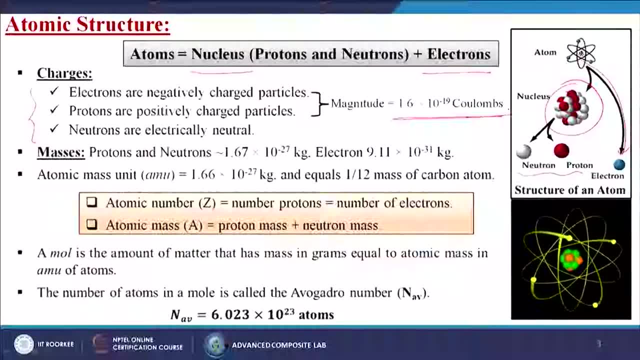 Generally, protons and neutrons masses are 1.67 into 10 to the power minus 27 kg. for electron, it is 9.11 into 10 to the power minus 31 kg. what is the atomic mass unit? or may be the AMU? 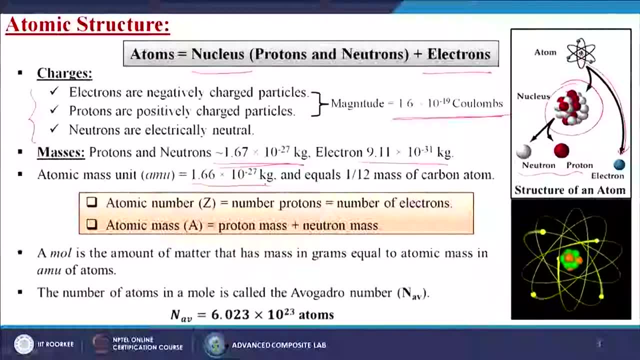 So generally it is 1.66 into 10 to the power minus 27 kg and equals to 1 by 12 mass of the carbon atom. so what is the atomic number Generally? it is generally denoted by number of protons, which is equal to number of the. 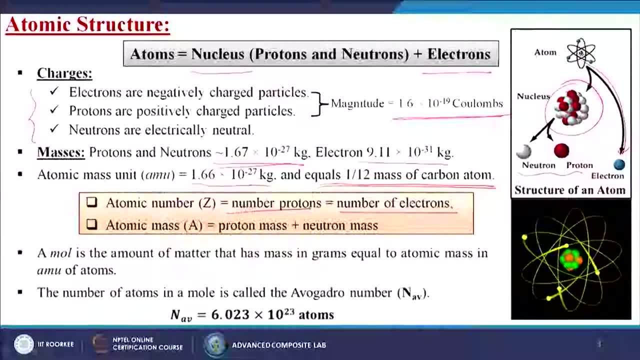 electrons. what is the atomic mass? So generally it is proton mass and the neutron mass. so a mole is the amount of matter that has mass in grams equal to atomic mass in grams. So what is the atomic mass? So what is the atomic mass? 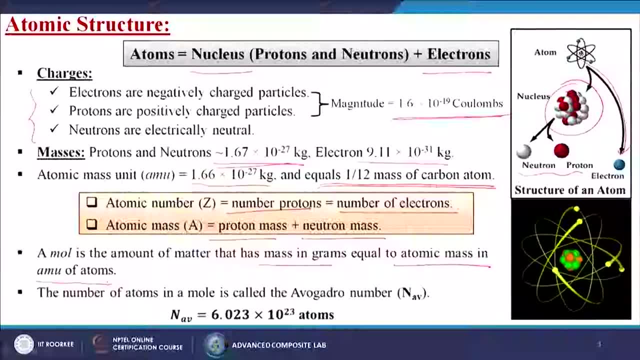 in AMU of atoms. so the number of atoms in a mole is called the Avogadro number. he is a famous scientist who discovered this numbers, and so the Avogadro number is 6.023 into 10 to the power 23 atoms. so first let us know the behavior of electron, so generally it 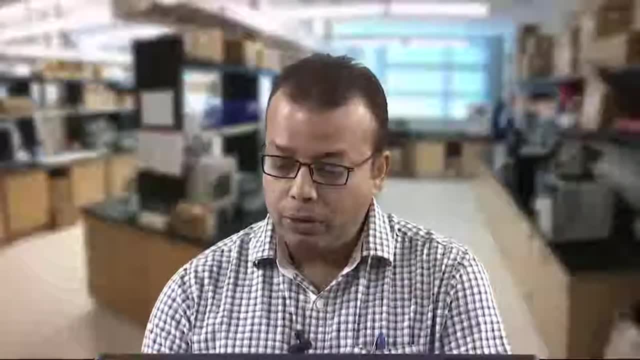 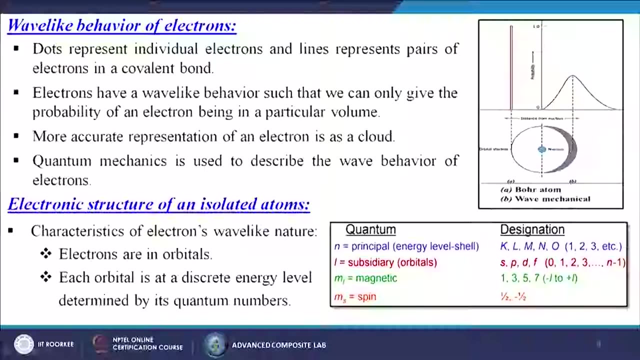 is a web like behavior. so dots, in this particular case, represents the individual electrons, and lines represents the pairs of electrons in a covalent bond. so in this case you can see some dots over there. so which is represent the individual electrons? so electrons have. 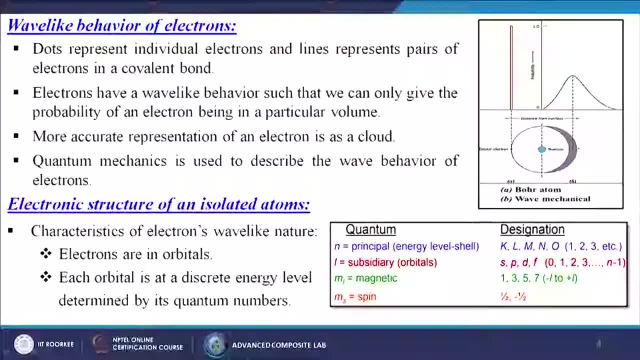 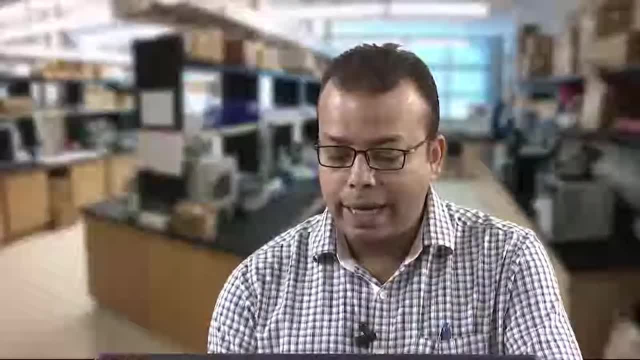 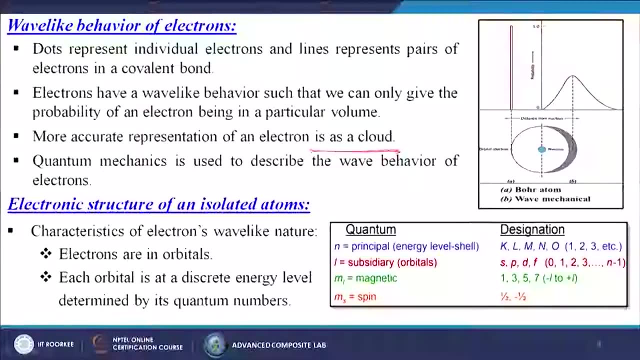 a web like behavior, such that we can only give the probability of an electron being in a particular volume. More accurate representation of an electron is as a cloud. quantum mechanics is used to describe the web behavior of electron. Generally electronic structure of an atom. 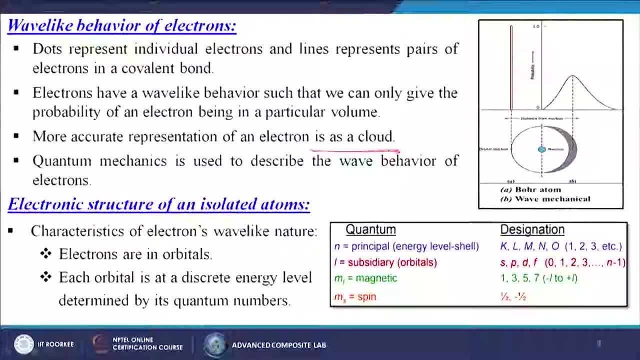 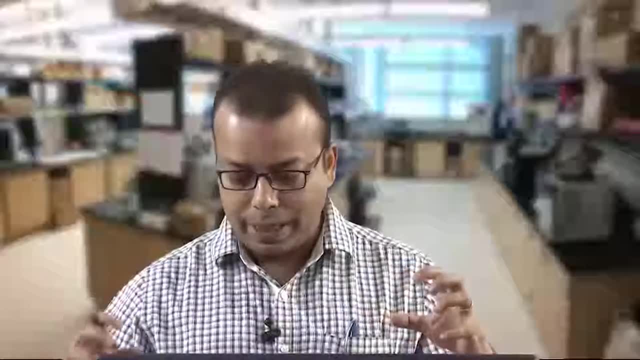 Isolated atoms. characteristics of the electrons web. like nature, electrons are in orbitals. each orbital is at a discrete energy level determined by its quantum number, so generally electrons are present, and then there is a gap, so the electrons are present in like. 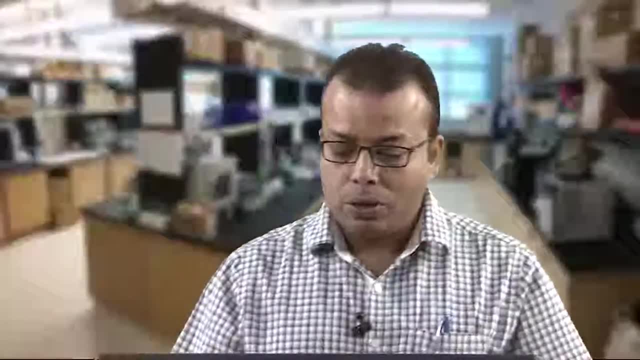 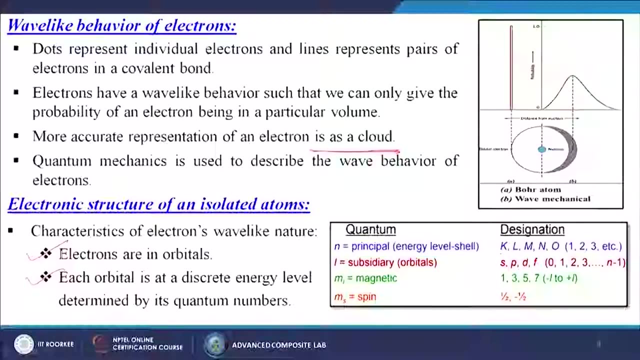 a orbital, it is like our galaxy. so what is quantum? So generally for n principle, energy level generally, we are giving the designations like K, L, M, N, Z. For I, subsidiary orbitals. generally it is S, P, D, F, generally 0,, 1,, 2,, 3, up to the 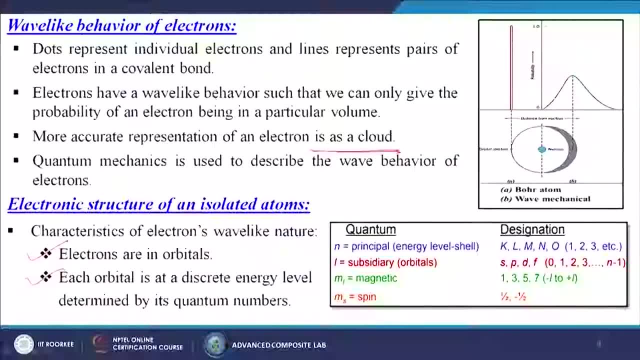 n minus 1, and for Mi magnetic it is 1,, 3,, 5,, 7, it is from minus i to plus i and M S pin. generally it is half or maybe the minus half. so these all are the different types. 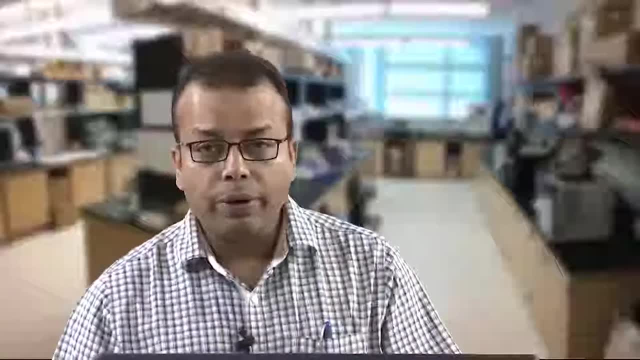 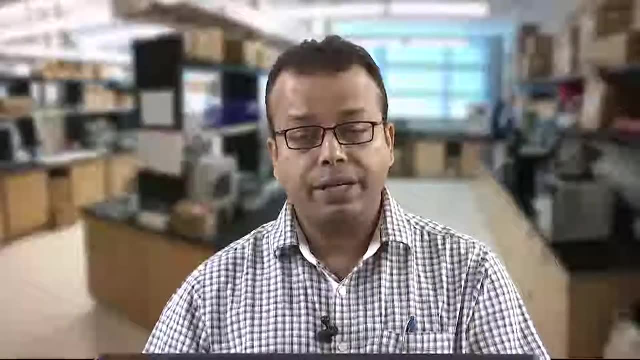 of electronic structure. So now we are going to discuss about the electronic structure of an electron. So now we are going to discuss about the electronic structure of an electron. So we have the electron energy states of isolated atoms. so electron have very discrete energy states, tends to occupy lowest available energy state unless 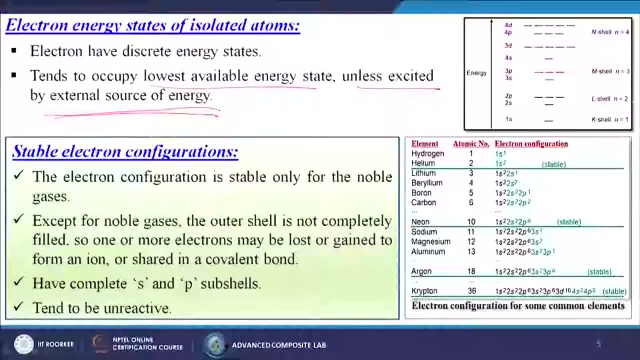 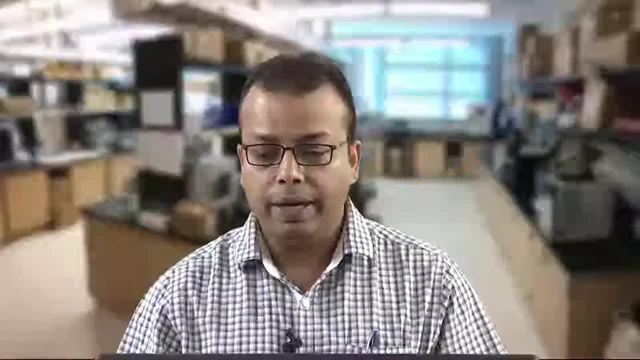 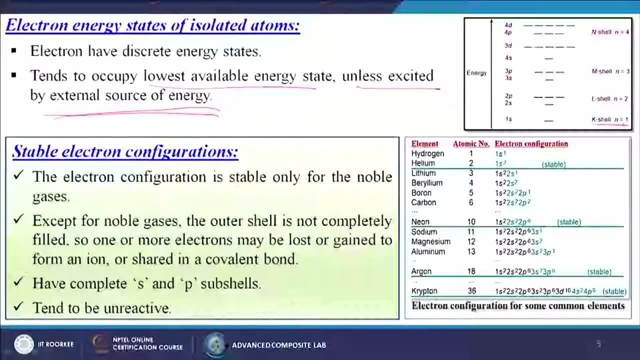 excited by the external source of energy. so we have to give the energy to the electron so that the electron can jump from the lower level to the higher level itself. so this is the energy level. so 1S. it is a K shell where N is equal to 1, and when we are increasing. 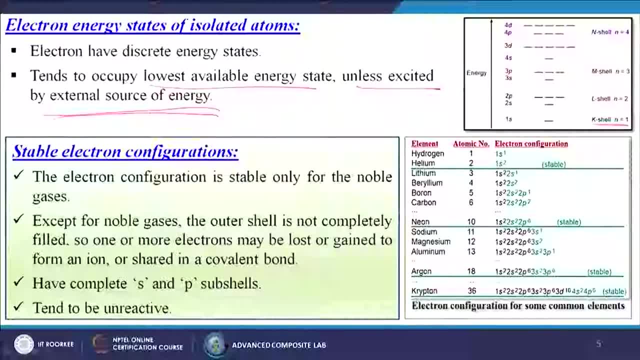 And when we are increasing the energy it is going to the up to the 4P or maybe the 4D, which is nth cell. that is, n is equal to 4, so what is the stable electronic configurations? The electron configuration is stable only for the noble gases, except for noble gases. 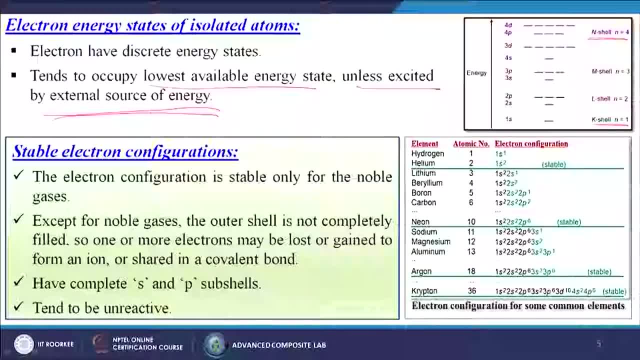 the outer shell is not completely filled because there is some vacancy, so one or more electrons may be lost or gained to form an ion or shared in a covalent bond, have complete S and P sub cells tend to be very, very unreactive. 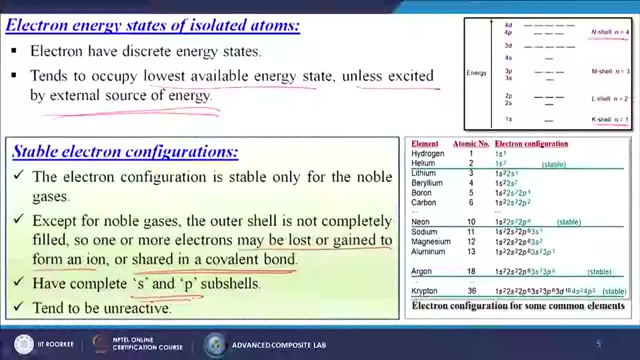 So here you can see the element and atomic number and the electronic configurations. so for hydrogen generally it is 1S1,, for helium it is 1S2, because atomic number is 2, so when we are talking about the say post carbon, so it is 6.. 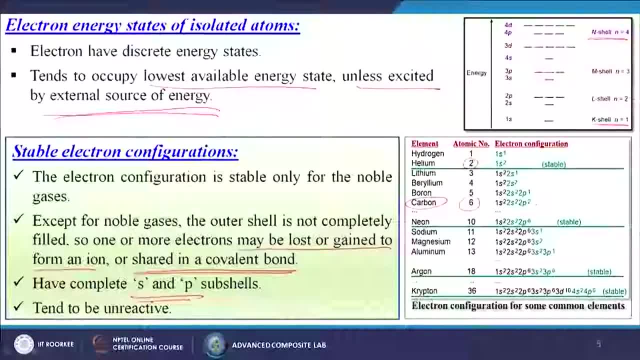 That means 1S2.. 1S2, 2S2 and 2P2, so it is total 6.. When you are talking about the magnesium, it is 12, 1S2, 2S2, 2P6 and the 3S2, when we 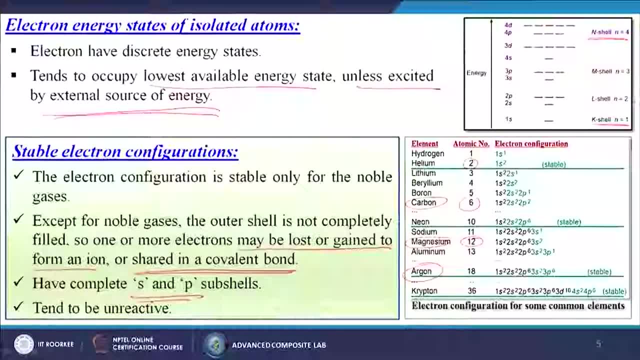 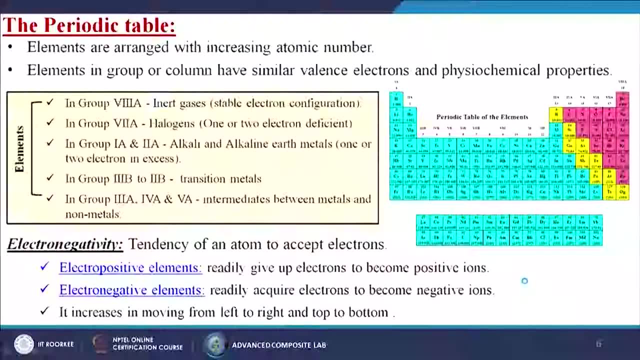 are talking about the argon. it is having 18 like 1S2, 2S2, 2P6, 3S2, 3P6, so it is shown. Now we are going to discuss about the periodic table, so elements are arranged with increasing. 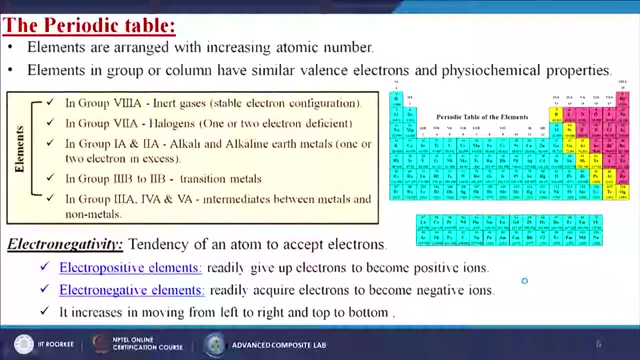 atomic number. elements in group or column have similar valence, electrons and the physiochemical properties, So elements in group 8A. so if we are talking about the 8,, so 8 group or maybe that 8A group, in this particular case it is inert gas, so stable electron configurations: helium, neon. 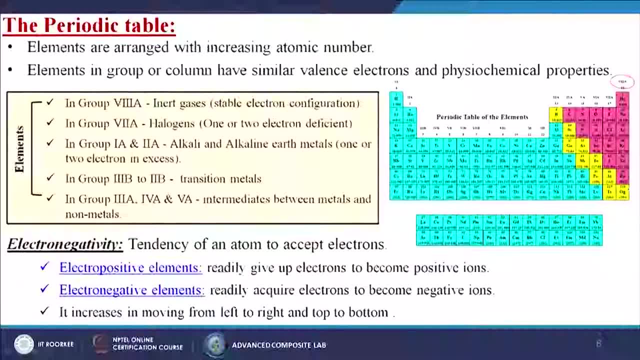 argon, krypton, xenon, radon and the OG, So in group 7A. so we are talking about the 7A. So here is the halogens. One or two electrons deficient are there? so, like for fluorine, chlorine, bromine, iodine? 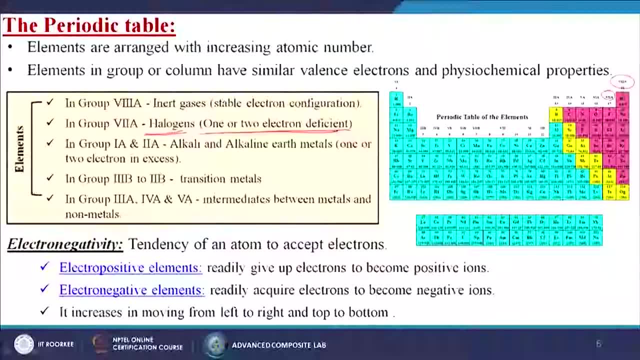 like that In group 1A and 2A. so when we are talking about 1A and 2A, alkali and the alkaline earth metals, one or two electrons in excess, like hydrogen, lithium, sodium, potassium, like. 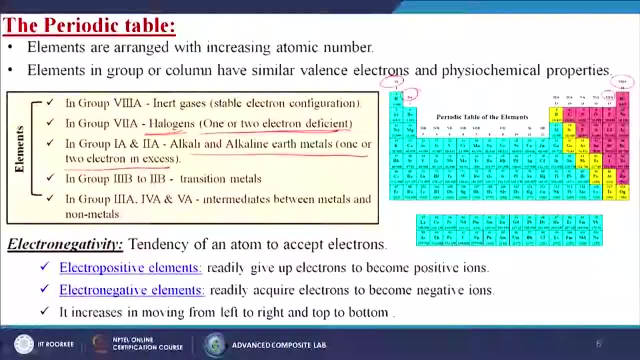 beryllium, magnesium, calcium, like that In group 3B and 2B. So generally here is the 3B and here is the 2B. So in this particular case these all are the transition metals, like strontium, like zinc. 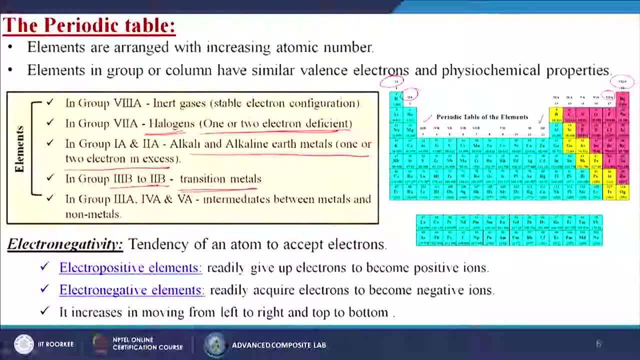 like cadmium, like mercury, so on, In group 3A, 4A and 5A. So in this particular case, the 3A, 4A and 5A, so this group, so it is the intermediates. 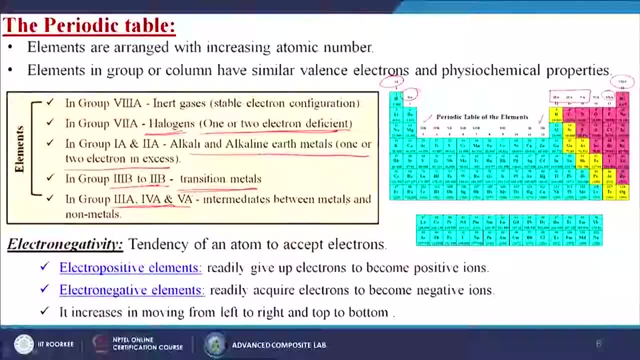 between metals and nonmetals Like boron, carbon, Carbon Nitrogen, or maybe aluminum, silicon, phosphorus, gallium, germanium, arsenic, so on. So what is the electronegativity? Tendency of an atom to accept electrons. that is why it became the negative. 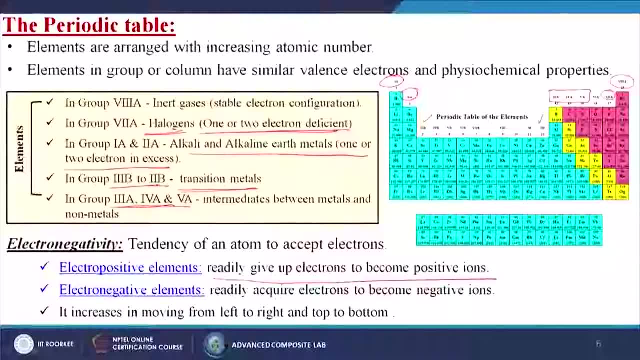 So electropositive elements readily give up electrons to become the positive ions, So it is losing the electrons. Electronegative elements readily acquire the electrons to become the negative ions, So it is accepting the electrons. It increases in moving from left to right and top to bottom. 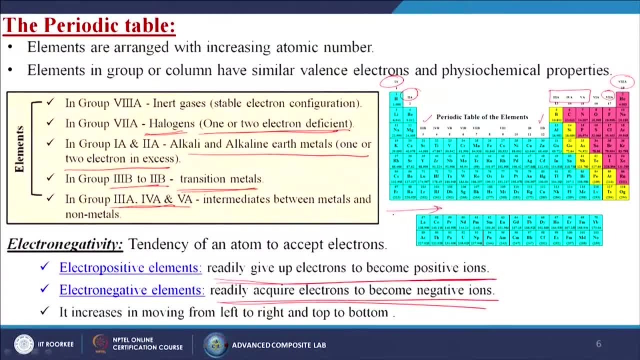 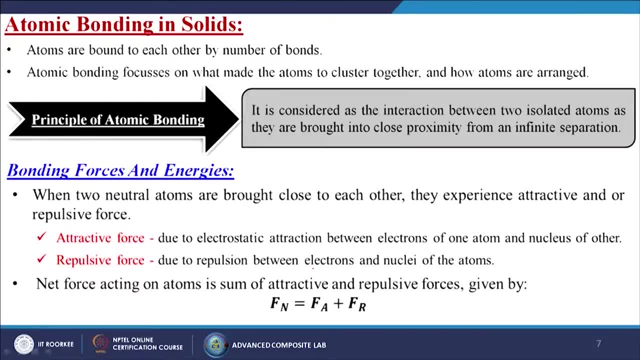 So it increases in the moving from from left to right and from the top to bottom. Now what is the atomic bonding in solids? So atoms are bound to each other by number of bonds, as we already know. So atomic bonding focus on what made the atoms to cluster together. 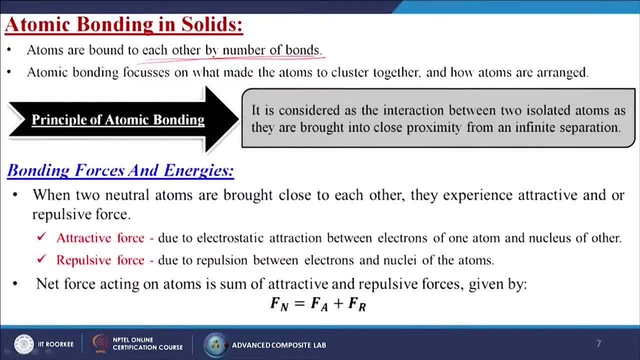 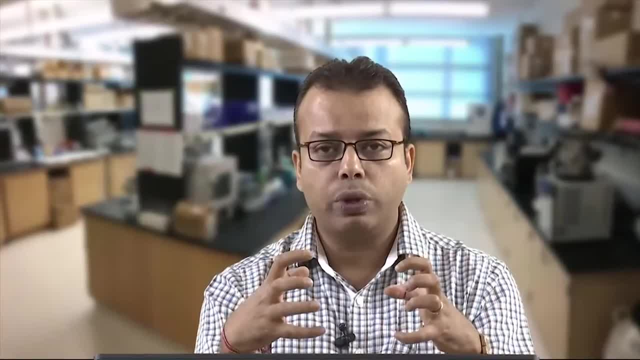 And how atoms are arranged. yes, as I told already, we are. we are having so many atoms, So there should be some bonding. then only the atoms can come close together and give a compact shape over there. So what is the principle of the atomic bonding? 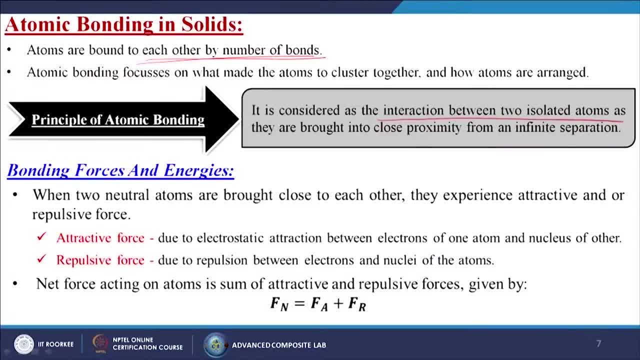 It is considered as the interactions between two isolated atoms as they are brought into close proximity from an infinite separations. So bonding force, and about their energies? So what is the bonding force? So when two neutral atoms are brought close to each other, they experience attractive. 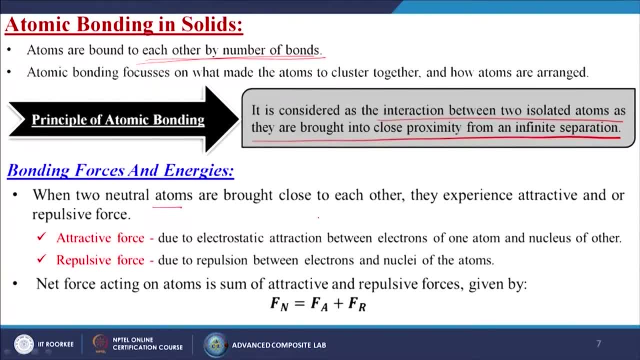 or maybe the repulsive force, as we know. So it is like a magnet, So attractive force. due to electrostatic attractions between electrons of one atom and nucleus of other. What is repulsive force? Due to the repulsion between electrons and the nuclei of the atoms itself. 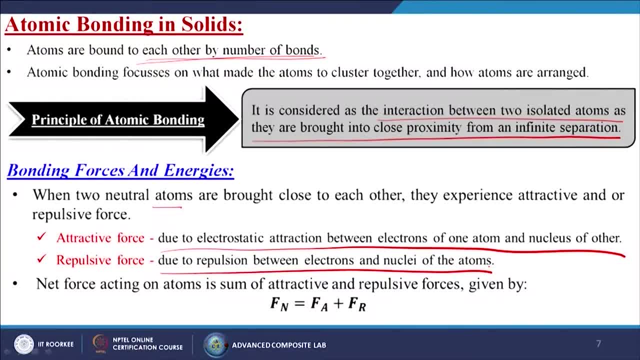 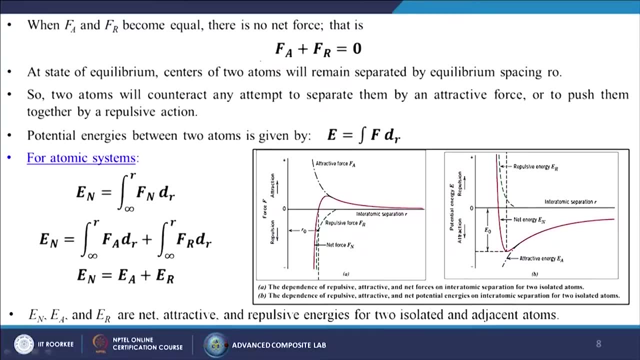 So net force acting on atom is some of the attractive and the repulsive force of course, which is given by F. net is equal to F attraction and the F repulsion. So when F, A and F R become equal there is no net force. that is F A plus F R is equal. 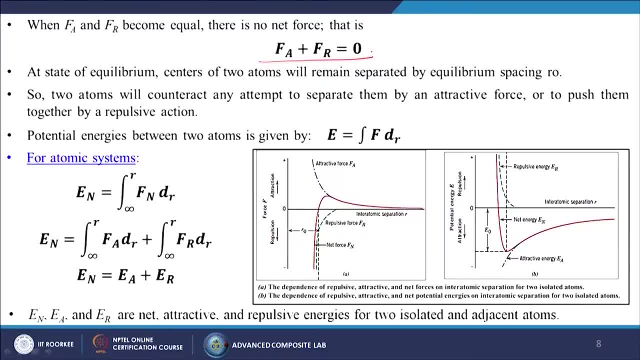 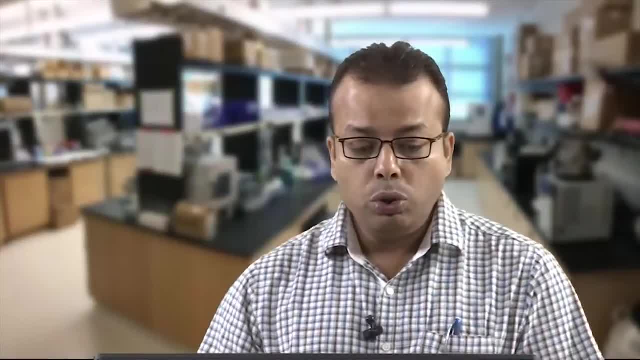 to 0.. So, as state of equilibrium, center of two atoms will remain separated by equilibrium spacing rho. So two atoms will counteract any at a to separate them by the repulsive force which is given by F. net is equal to F attraction and the repulsive force. 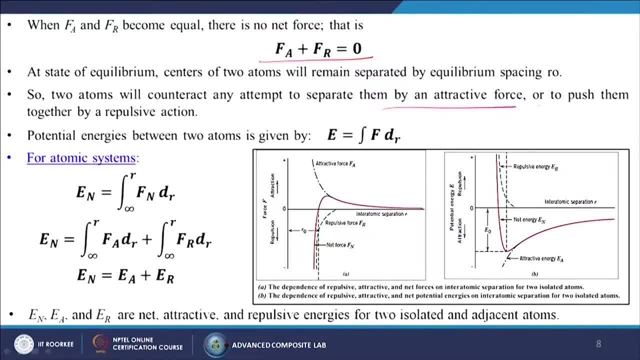 So when F A and F R become equal there is no net force, that is F A plus F R is equal to zero, an attractive force or to push them together by a repulsive action. so potential energy between two atoms is given by. E is equal to integration FDR. so for atomic systems generally, 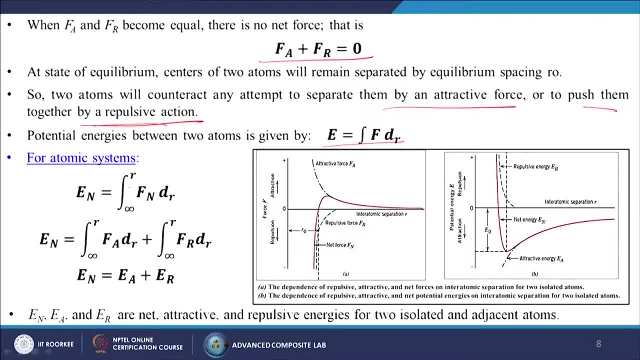 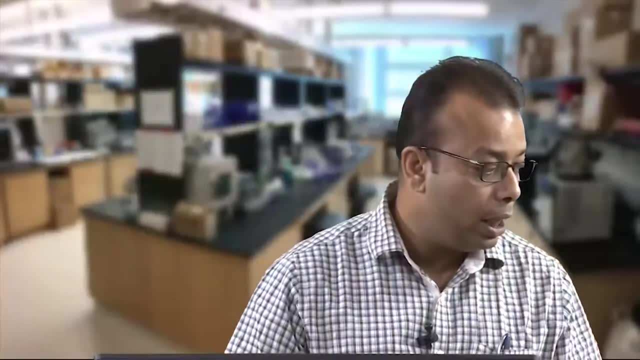 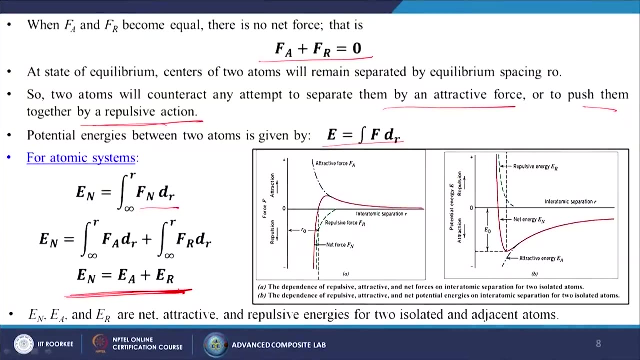 EN is equal to integration infinity to R FNDR, which is nothing but the integration infinity to R FADR plus integration infinity to R FRDR, because for the attraction and for the repulsion force that means EN is equal to EA plus ER. so here EN, EA and ER are net attractive. 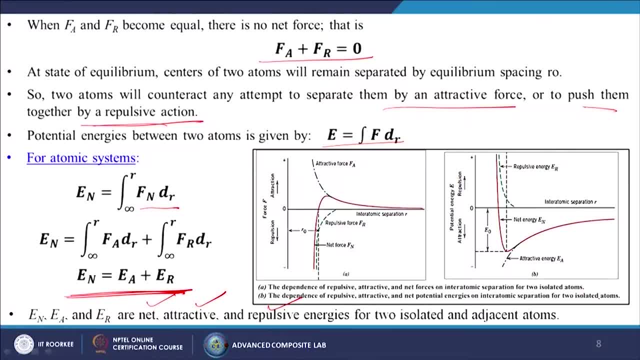 and the repulsive energies for two isolated and the adjacent atoms. so in this particular case you can see that atomic force is infinite. this particular case, and then the repulsive force, and then we are getting the net force here in this particular line. so this is known as the RO. so if we put a tangent over there, 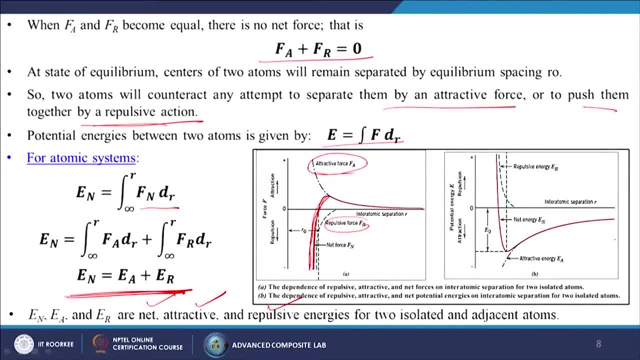 so in this particular case also so. this is generally for the dependence of the result repulsive, attractive and net force on interatomic separations for two isolated atoms. here the dependence of repulsive, attractive and net potential energies on interatomic separations for two isolated atoms. 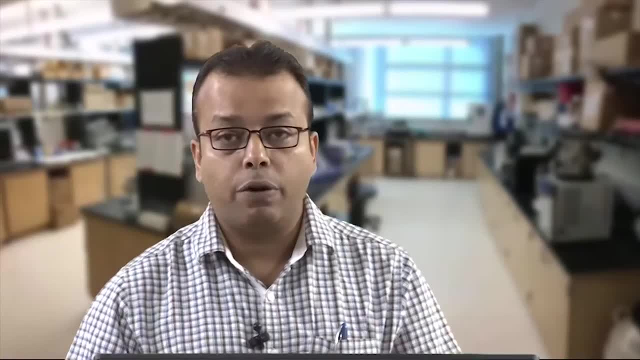 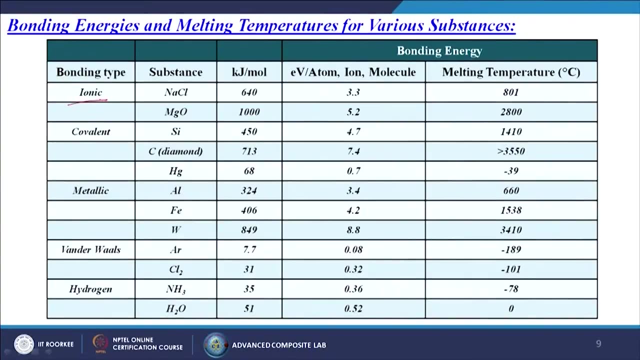 So now we are going to discuss about the bonding energies and melting temperature for various substances. so generally bonding type, we are going to know that ionic for, like sodium chloride or maybe the magnesium oxide, same, what is the electron volt per atom? or ion or maybe? 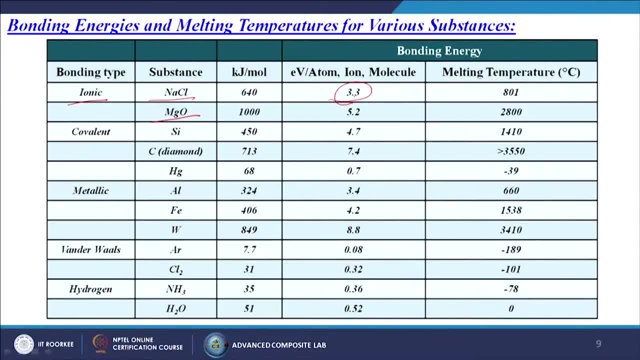 the molecule. The bonding energy? it is 3.3,. what is the melting temperature? It is 801,, when we are talking about the covalent bond, generally silicon, or maybe the carbon, so its bonding energy is 4.7 and melting temperature is 1410, for carbon, it is 7.4 and it is more. 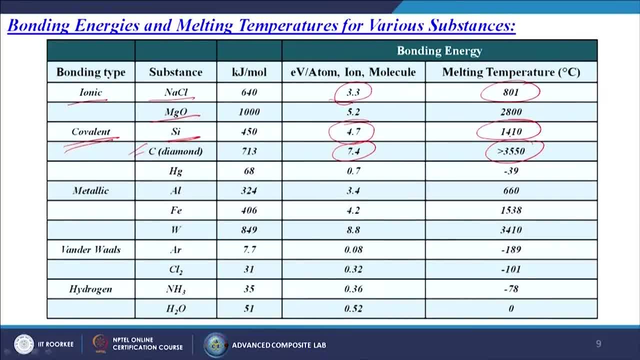 than 3550,. when we are talking about the metallic, so for the generally, the metals, metallic bonding. so metallic bonding, like ammonium, it is 3.4, its melting temperature is more than 660 degree centigrade. when we are talking about the van der Waals bonding, or maybe the van der Waals 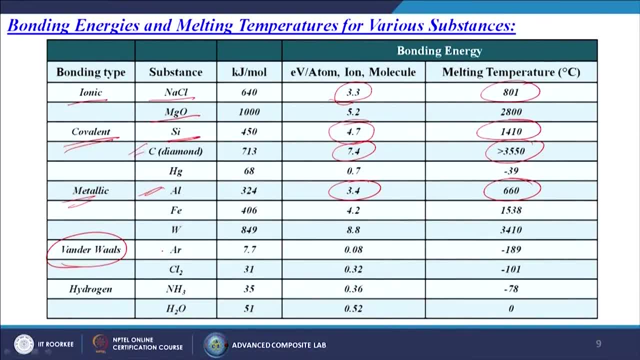 interactions. so generally for argon, it is 0.08 and the melting temperature is minus 189, it is very, very weak bonding. When we are talking about the hydrogen bonding generally for the ammonia, we are getting it 0.36 and the melting temperature is 0.38. 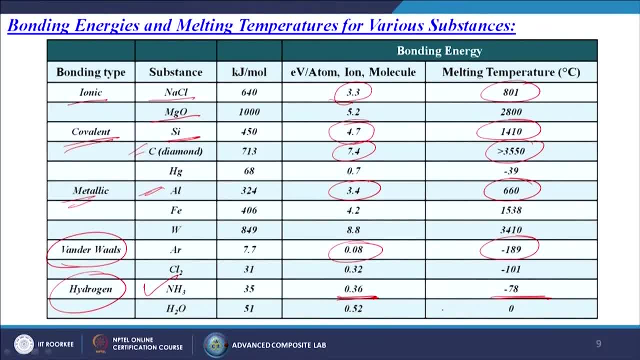 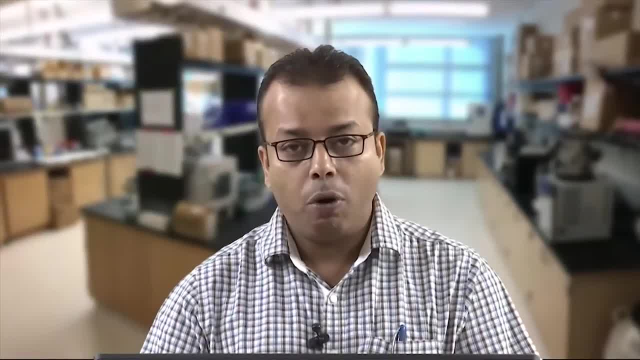 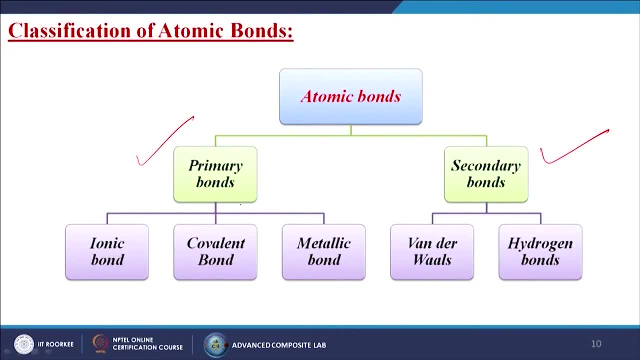 Okay, The melting temperature is minus 78. So now we are going to briefly discuss about the atomic bonds. so generally, the atomic bonds has been divided into two parts. one is called the primary bonds, another one is called the secondary bonds. So primary bonds is divided into three parts, that is, ionic bond, covalent bond and the. 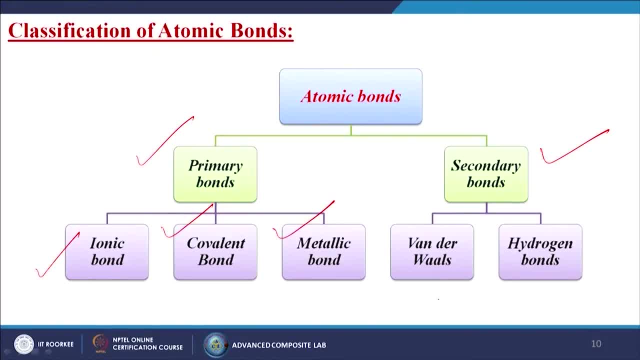 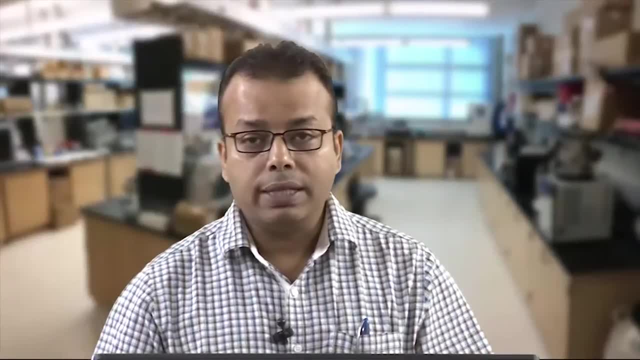 metallic bond and secondary bonds is two types. one is called the van der Waals bonds or maybe the interactions, another one is called the hydrogen bonds. So what is the interatomic bonds? So primary bonds, generally ionic, covalent and metallic bonds, are relatively very, very 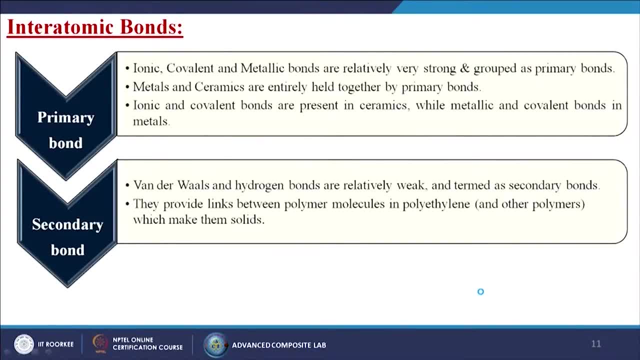 strong and grouped as primary bonds. So metals and ceramics are entirely held together by the primary bonds itself. Ionic and covalent bonds are present in ceramics, while metallic and covalent bonds in metals. So when we are talking about the secondary bond, generally- van der Waals and hydrogen- 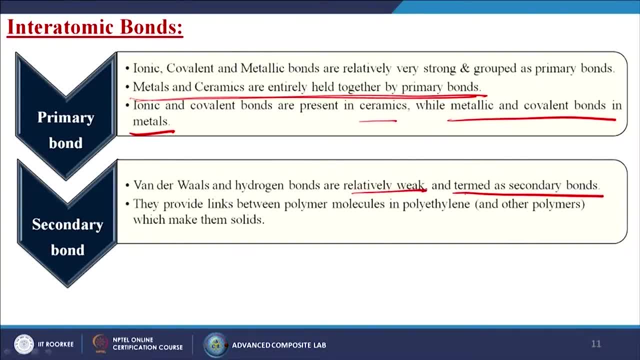 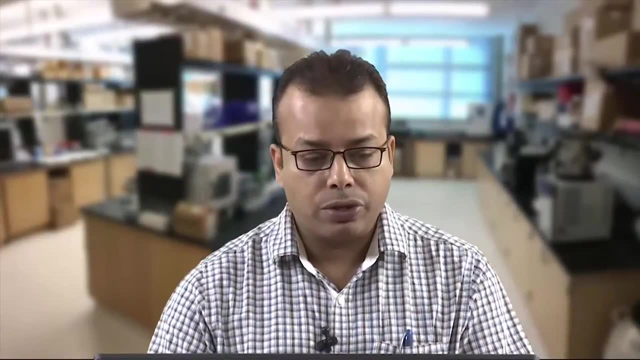 bonds are relatively weak, termed as the secondary bonds, as I told already. they provide links between the polymer molecules in polyethylene and other polymers which make them solid. So now, first we will discuss about the ionic bonds. so it exists between two atoms when 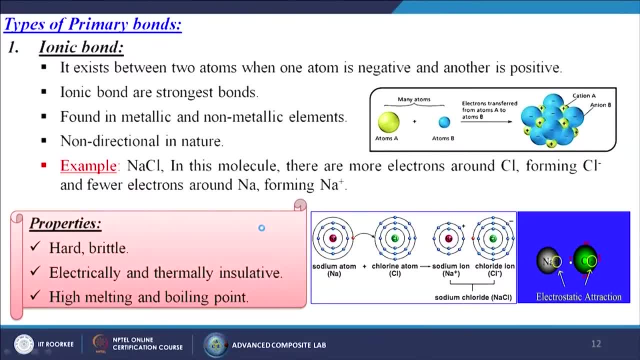 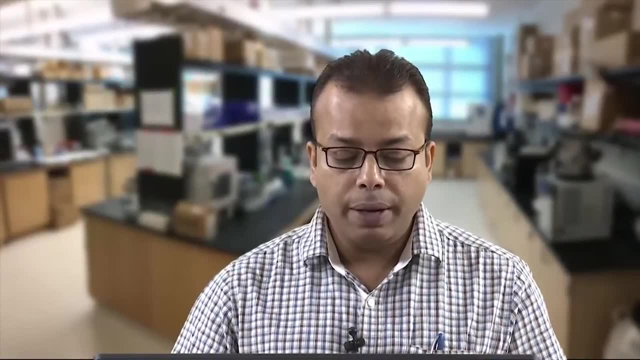 one atom is negative and another is positive. ionic bonds are the strongest bond found in metallic. Ionic bonds are non-metallic elements, non-directional in nature, so like the best example is that salt sodium chloride, so sodium chloride. in this molecule there are more electrons. 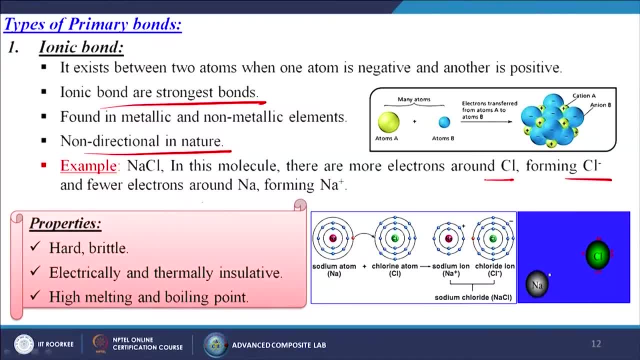 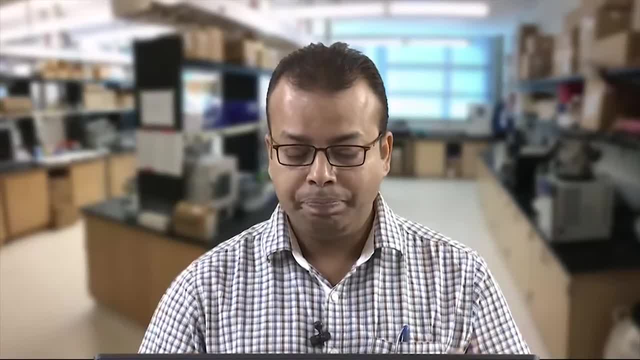 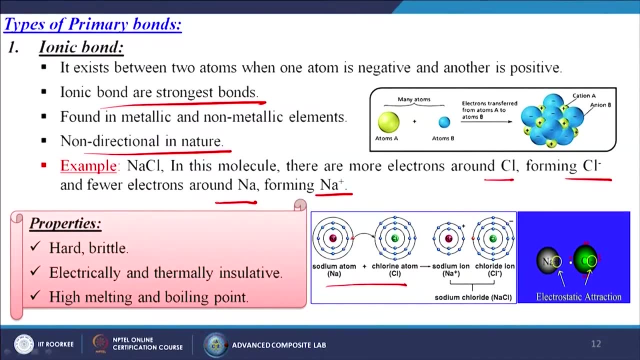 around chlorine, forming Cl minus, and fewer electrons around sodium, forming the Na plus. so Na plus and Cl minus positive and negative. So in this particular case, when the sodium is reacting with the chlorine, so excess electron is jumping onto the chlorine atom and sodium became the Na plus and the chlorine became 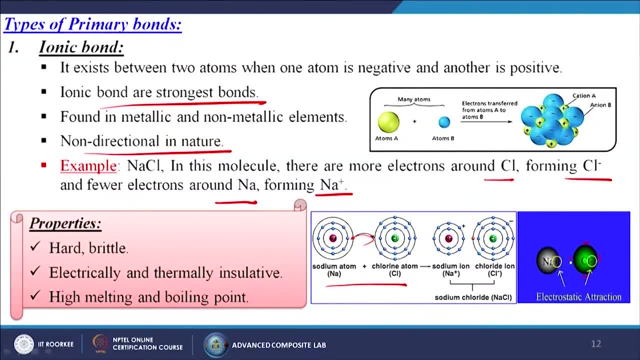 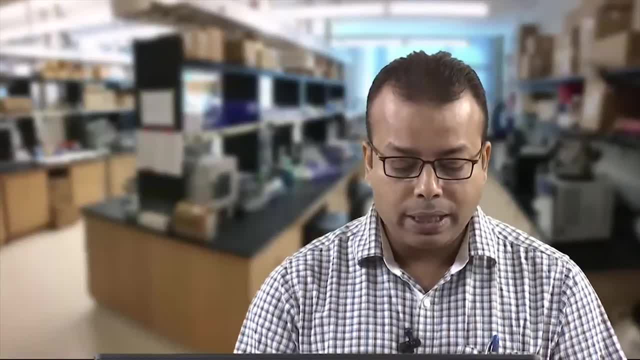 the Cl minus. so it is like that. so Na plus and the minus. some electrostatic attraction is taking place in between that. What is the properties? It is very, very hard, brittle in nature, electrically and thermally insulative, high melting and 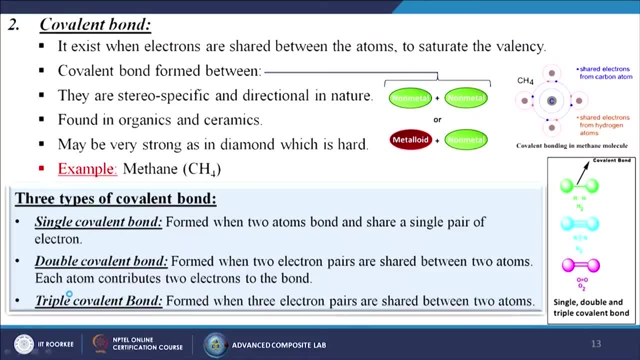 the boiling point. Now we are going to discuss about the covalent bond. It exists. Covalent electrons are shared between the atoms to saturate the valency covalent bond formed between non-metal, or maybe the non-metal, or maybe the metalloid and non-metal. 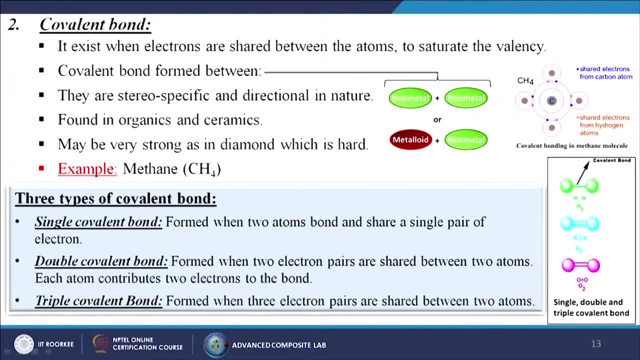 They are stereospecific and directional in nature, found in organics and ceramics, maybe very strong, as in diamond, which is very, very hard. example is the methane, CH4, so in this particular case, You can see that C is present in this main orbital and then H is surrounded by this and 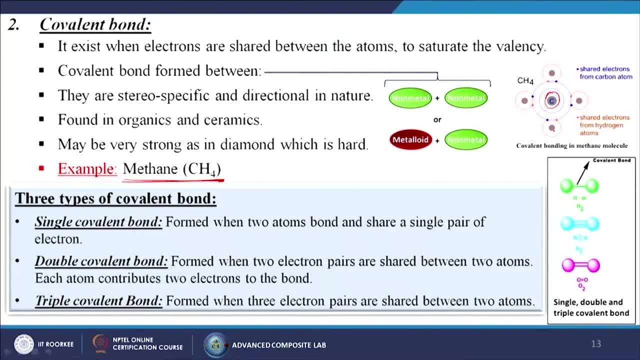 this. all are attached with the covalent bonds. So three types of covalent bonds. first one is called the single covalent bond, formed when two atoms bond and share a single pair of electrons. next, double covalent bond, formed when two electrons pair or share between two atoms. each atom contribute to two electrons. 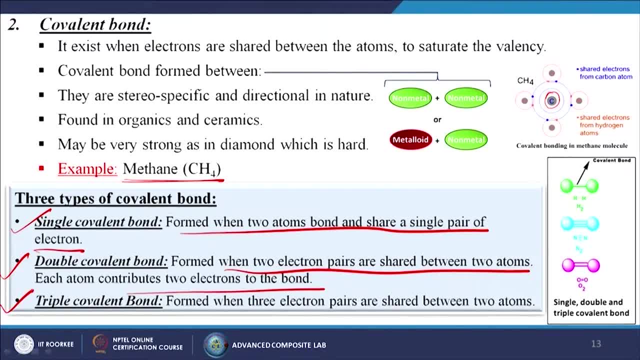 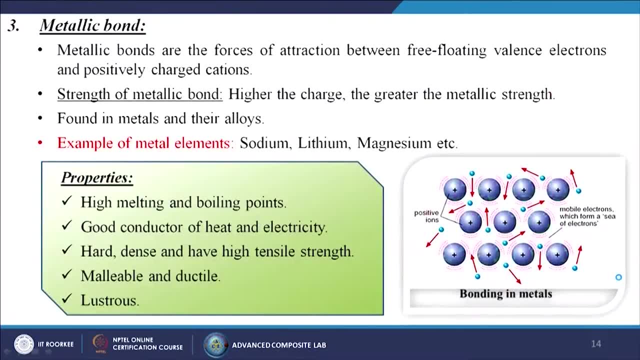 to the bond. And the third one is that triple covalent bond formed when three electrons pairs are shared between two atoms. Now we are going to discuss about the metallic bond. metallic bonds are the forces of attractions between free floating valence electrons and positively charged cations. strength of metallic 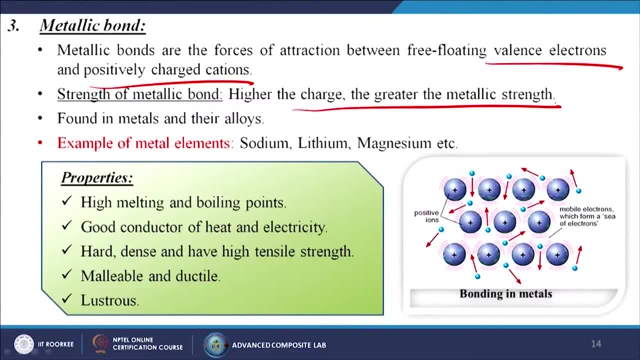 bond. higher the charge, the greater the metallic strength found in metals and their alloys. example of metal elements Like sodium, lithium, magnesium. so what are the properties? Like high melting and boiling points, good conductor of heat and electricity, hard dense and have tensile strength, malleable and ductile. and it is very, very lustrous means glittering. 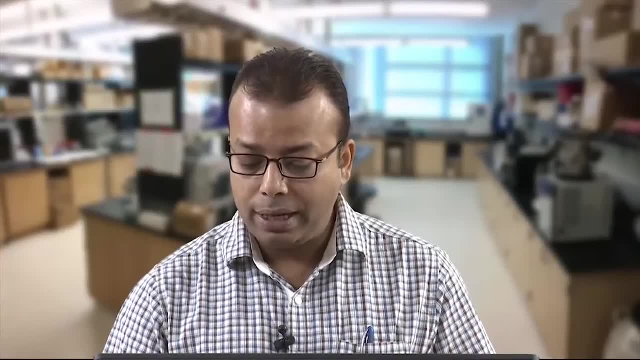 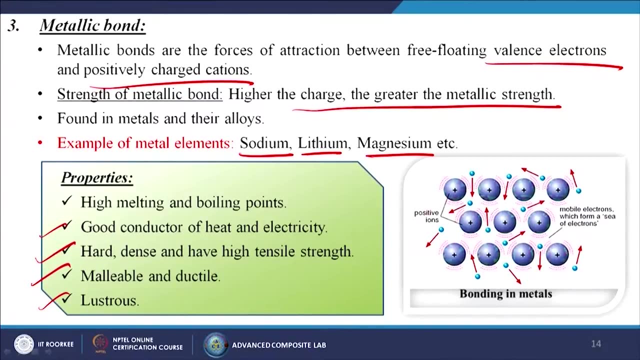 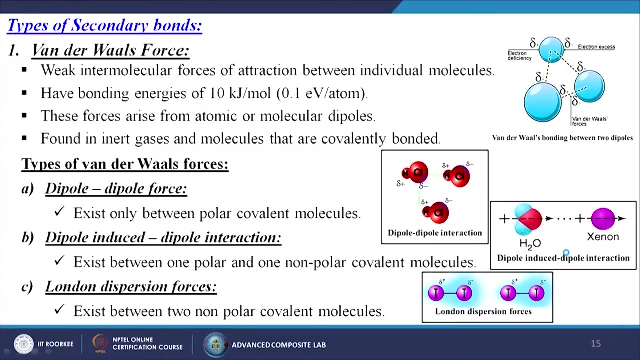 in nature. So here are the bondings in the metals. so due to that ions, so generally the bonding are taking place And that should be the charged cations. So now we are going to discuss about the types of secondary bonds. first it is the van der. 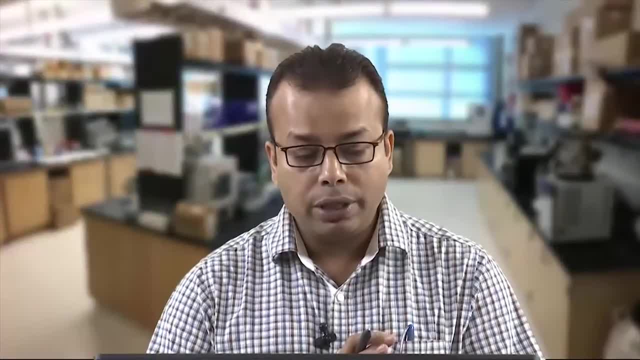 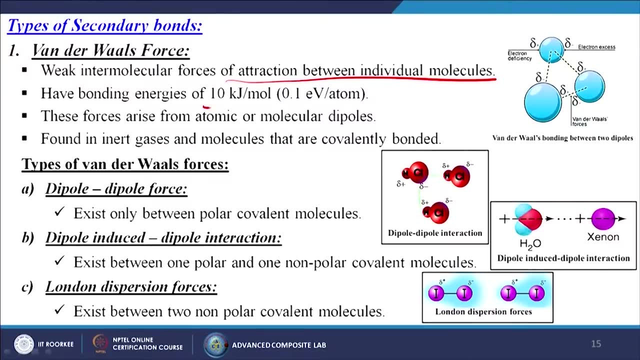 Waals force. it is a very, very weak. already I told you the weak intermolecular forces of attractions between the individual molecules have bonding energies of 10 kilo joule per mole. it is equivalent to 0.1 electron volt per atom. these forces arise from atomic or 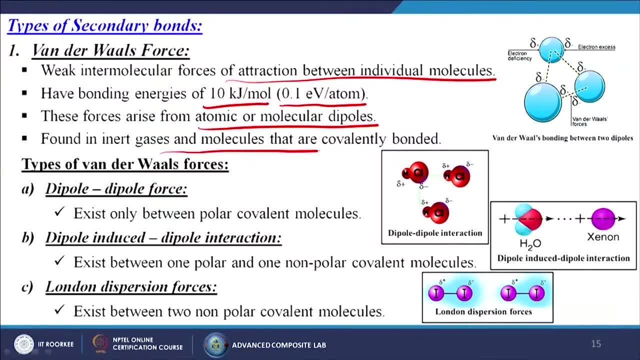 molecular dipoles Found in inert gas and molten gas, Inert gas and molecules that are covalently bonded. So there are three types of generally van der Waals forces. first one is called the dipole-dipole force exist only between polar covalent molecules. 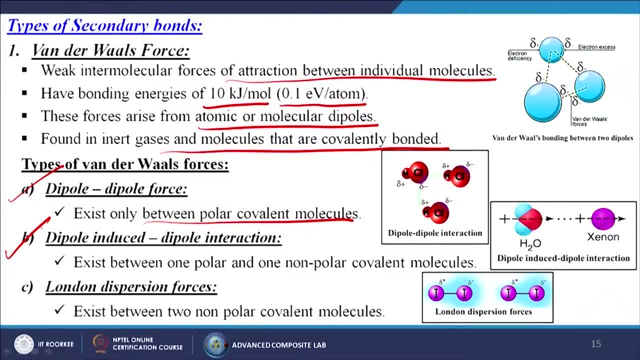 Second is dipole induced. dipole interaction exist between one polar and one non-polar covalent molecules, And the last one is called the London dispersion forces exist between two non-polar covalent molecules. So this is the London dispersion. 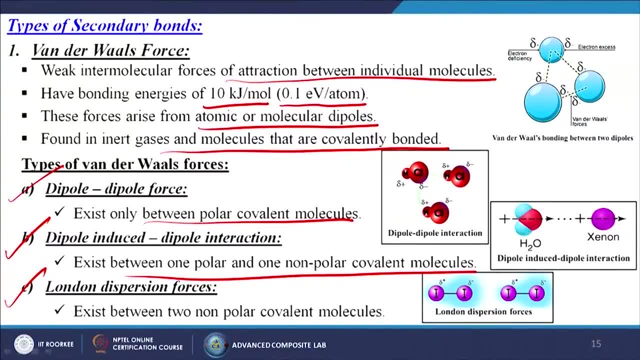 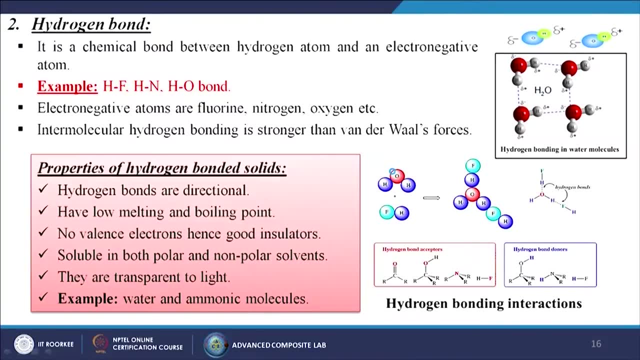 So in this particular case you can see that two non-polar covalent molecules and in between that It is the dipole induced interactions example and it is the dipole-dipole interaction. Next we are going to discuss about the hydrogen bond. it is a chemical bond between hydrogen. 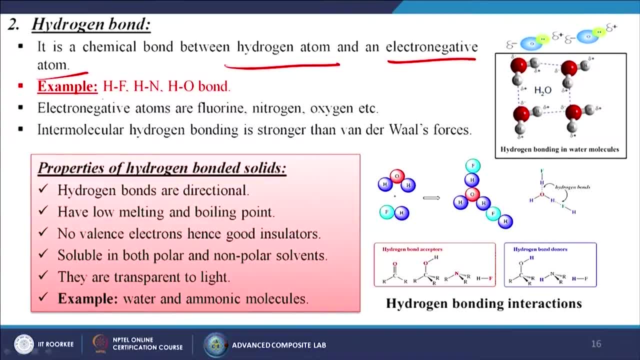 atom and an electronegative atom. generally we can find it like HF, HN, HO bond. generally it is called the hydrogen bond, Electronegative atoms. Electronegative atoms, Electronegative atoms are fluorine, nitrogen, oxygen. intermolecular hydrogen bonding is 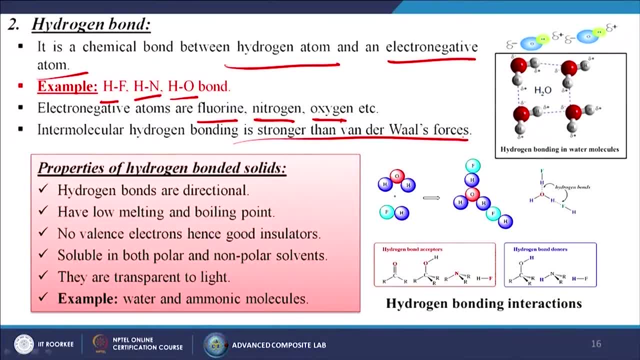 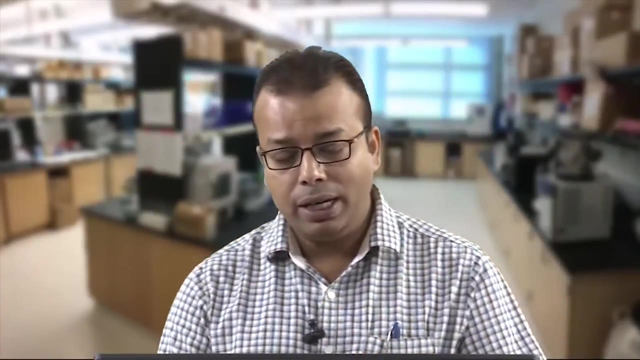 stronger than the van der Waals force. So properties of the hydrogen bond. so hydrogen bonds are directional, so have low melting and boiling point. no valence electrons, hence good insulators. so soluble in both polar and the non-polar solvents. they are transparent to the light. example, best example is the water. 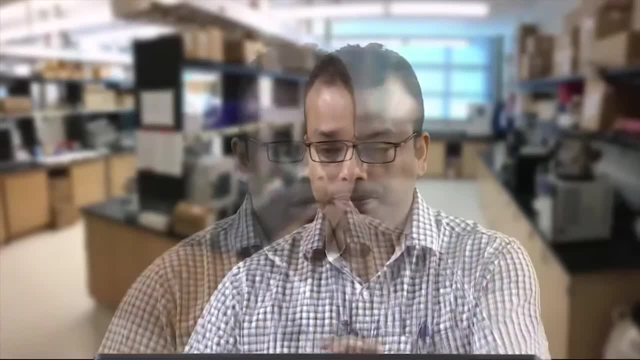 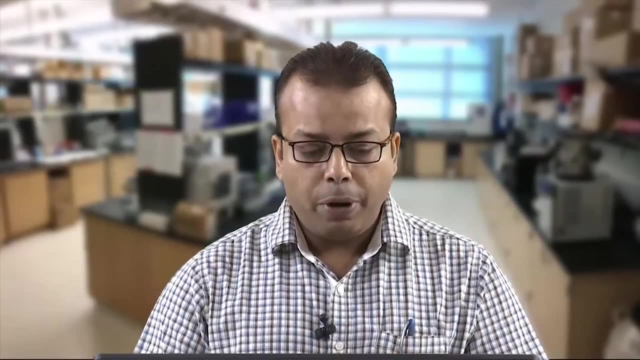 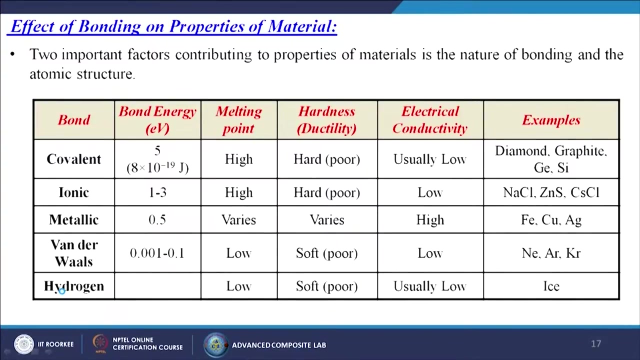 and the some ammonic molecules. So now we are going to discuss about the effects of bonding on the properties of materials, how it affects two important factors contributing to properties of materials is the nature of bonding and, of course, the atomic structure. So first we are going to discuss the covalent bond. so bond energy is 5 electron volt melting. 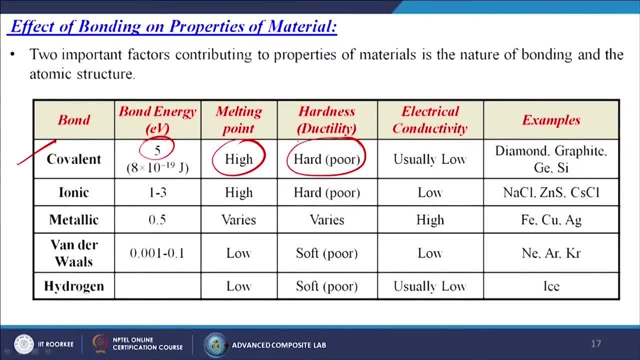 point is high. hardness in terms of ductility: it is hard and ductility is very, very poor. electrical conductivity usually low, and the examples: diamond, graphite, germanium, silicon. it is ionic generally the bond energy is 1 to 3, melting point is high. it is hardness. 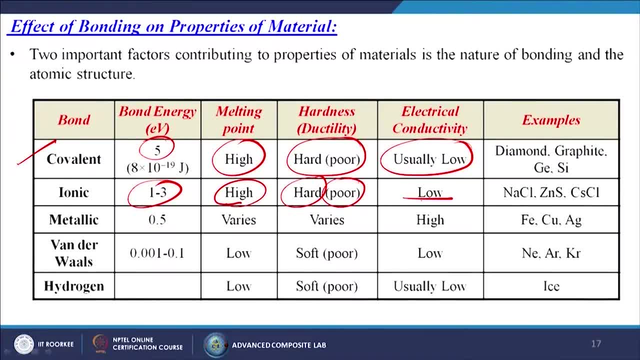 is hard. ductility is very, very poor. electrical conductivity is low, like sodium chloride, zinc, sulphide and the CSCL. So when you are talking about the metallic, it is 0.5 electron volt. it is melting point. 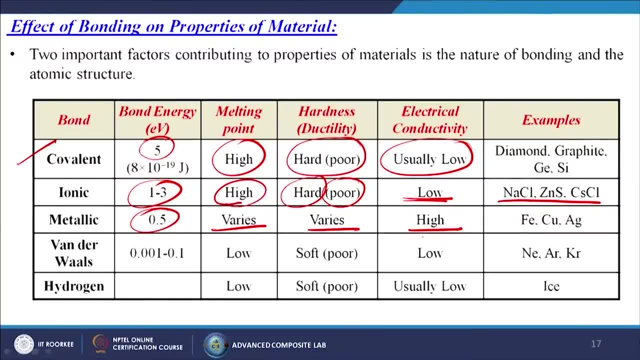 varies, hardness also varies And electrical conductivity is very, very high, like iron, copper, silver, etc. Van der Waals force: it varies from 0.001 to 0.1, melting point is low, then hardness is soft, but ductility is also very poor. electrical conductivity is also low, like 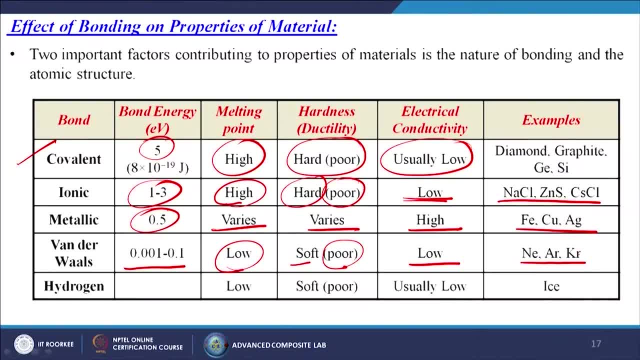 neon, argon, krypton, like that. And last one is the hydrogen. its melting point is very, very low, hardness is soft and ductility is poor, Usually low and generally the example is the ice or maybe the water. 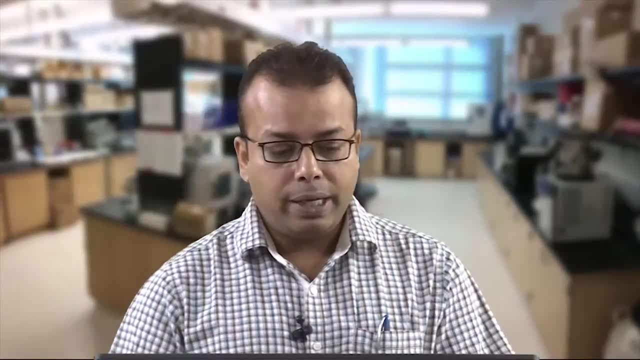 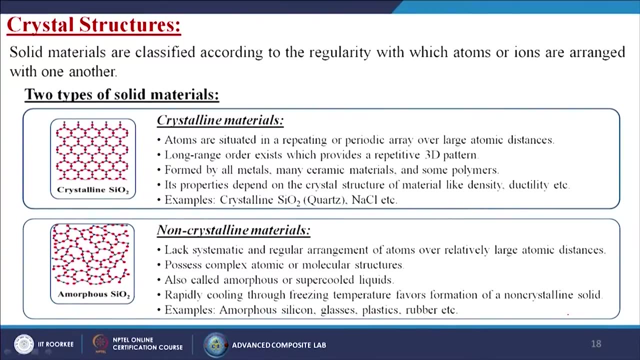 Now we are going to discuss about the crystal structure. So solid materials are classified according to the regularity with which atoms or ions are arranged with one another. Two types of solid materials generally. one is called the crystalline materials, another one is called the non-crystalline materials. 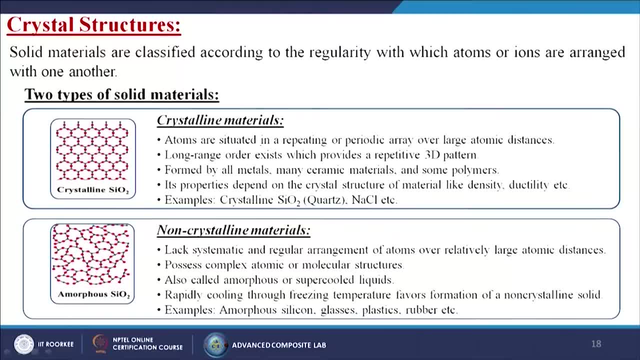 So what is the crystalline materials? Atoms are situated in a repeating or periodic array over large atoms. Let me give you a few examples. So the crystalline materials are classified according to the regularity with which atoms are arranged with one another. 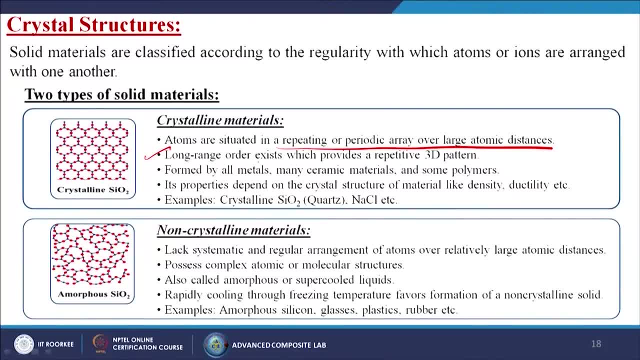 atomic distances long range order exist which provides a repetitive 3D pattern formed by all metals, many ceramic materials and some polymers. its properties depend on the crystal structure of materials, like density, ductility, etcetera. examples: crystalline silicon. dioxide. 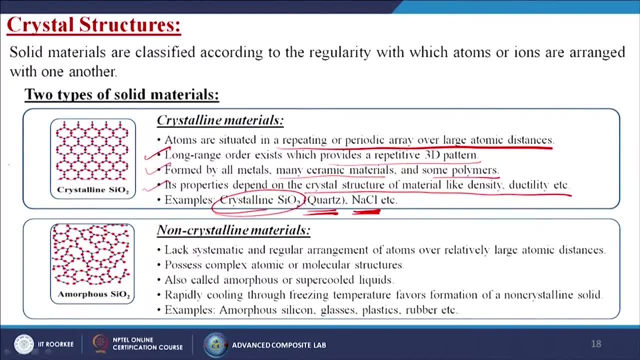 generally known as quartz sodium chloride. so you can see the crystalline silicon dioxide crystal structure. Then we are going to discuss about the non-crystalline materials. so it's having very lack systematic and regular arrangement of atoms over relatively large atomic distances. possesses complex 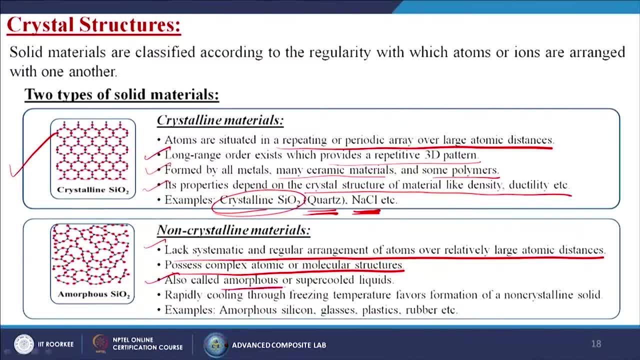 atomic or molecular structures, also called the amorphous or maybe the supercooled liquids. rapidly cooling through freezing temperature favors formation of a non-crystalline solids. what is the example? Amorphous silicon, glasses, plastics, rubber plastic. 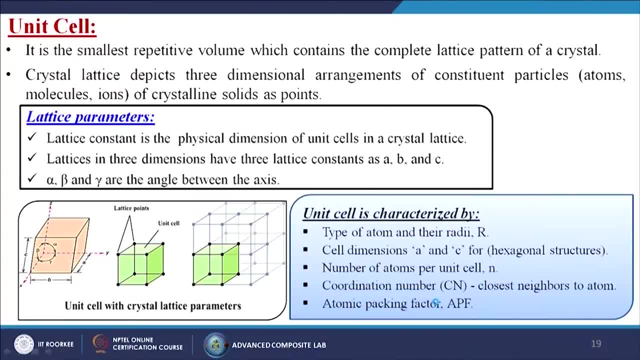 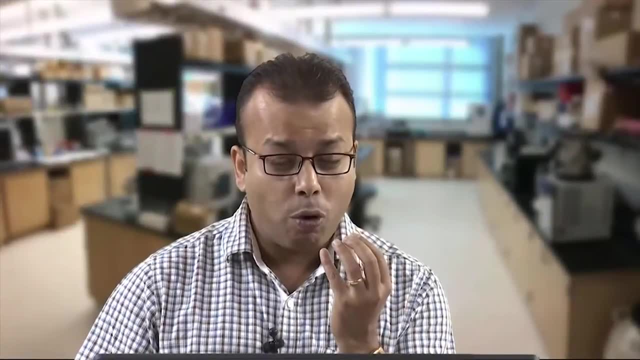 Okay, Etcetera. Now we are going to discuss one very interesting thing that is called the unit cell. so it is the smallest repetitive volume which contains the complete lattice pattern of a crystal. so it is the one, you can say one small backbone kind of things. so crystal lattice depicts. 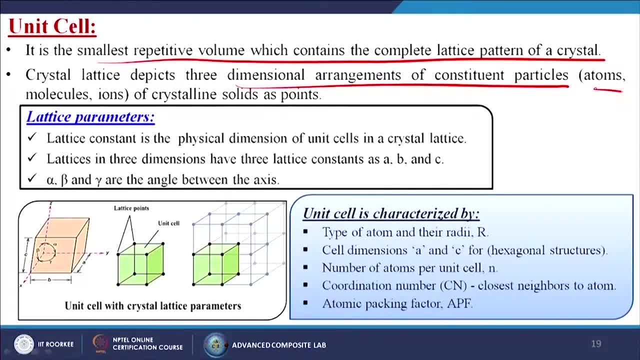 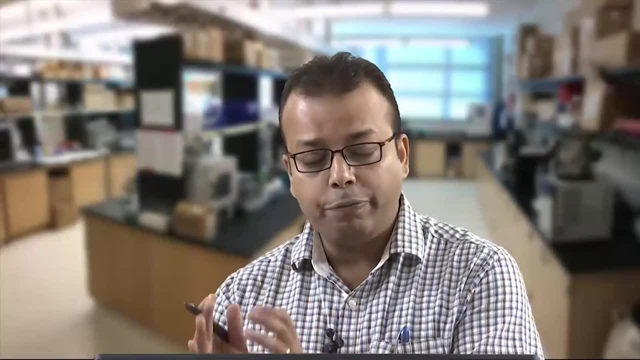 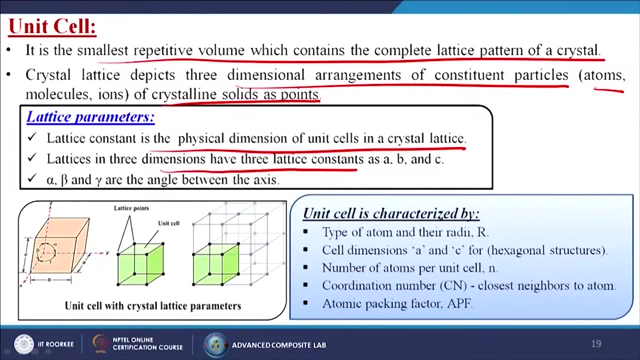 three dimensional arrangements of constituent particles like atoms, molecules and the ions of crystalline solids as point Lattice parameter. lattice constant is the physical dimension of unit cell in a crystal lattice. this part I will briefly discuss in the subsequent lecture. Lattice in three dimensions have three lattice parameters like A, B and C: alpha, beta and 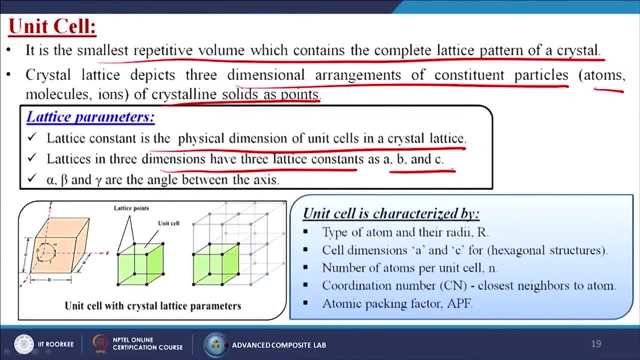 gamma are the angle between the axis. so if you see the lattice parameters- so here this angle is alpha- then this is beta and gamma. Okay, And this is the gamma one. so lattice point, this is the unit cells. so this is denoting: 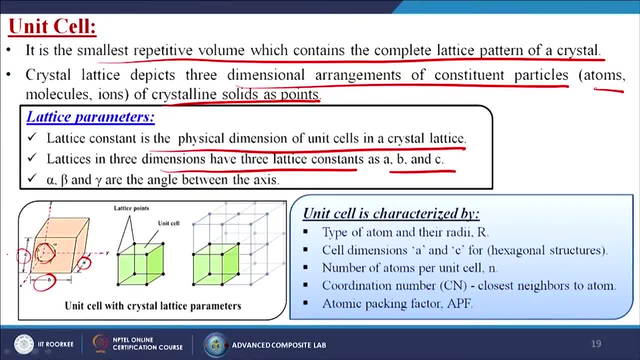 by A, this is B and this is C. if it is the cubic one, then A is equal to B is equal to C. So generally, unit cell is characterized by type of atom and their ready are cell dimensions, A and C for the hexagonal structures. number of atoms per unit cell, that is N coordination. 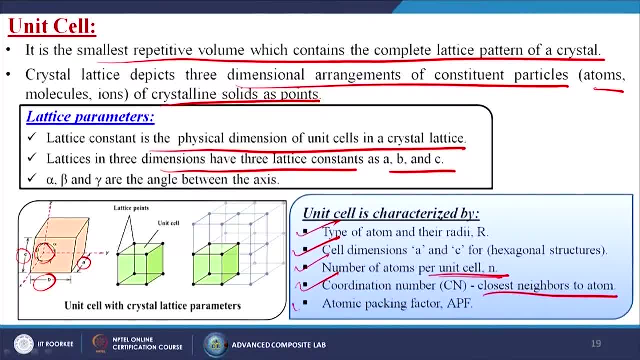 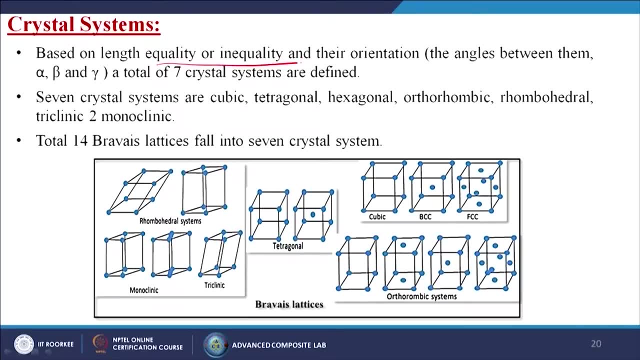 number. This is the closest number to atoms and atomic packing factor, that is, APF. this all, in brief, I am going to discuss into the second lecture. So what is crystal systems Based on length, equality or inequality, and their orientations, the angles between them. 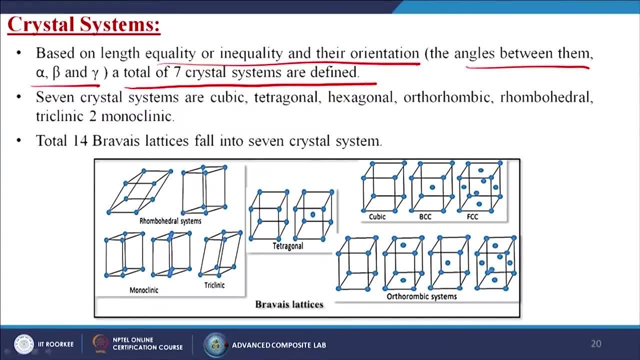 alpha, beta and gamma. a total of seven crystal systems are defined. seven crystal systems are cubic, tetragonal, hexagonal, orthorhombic, rhombohedral, triclinic to monoclinic. Total 14 Bravais lattice fall into seven crystal systems. 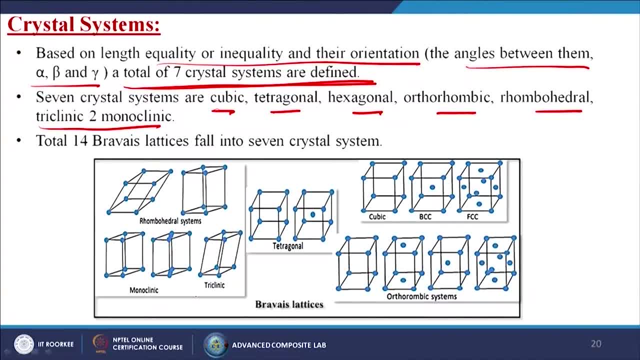 So this is the example of the rhombohedral systems: monoclinic and the triclinic, then tetragonal, then cubic, like BCC, body centered cubic, FCC, face centered cubic. this is the orthorhombic systems. 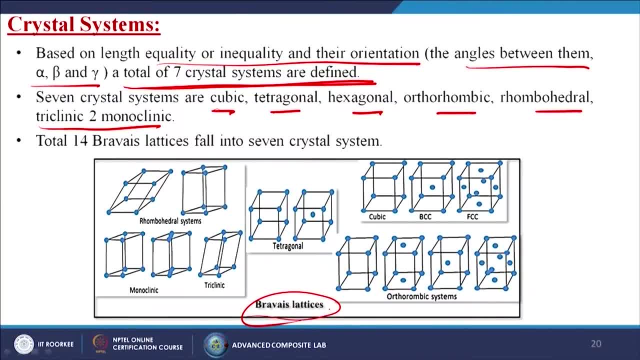 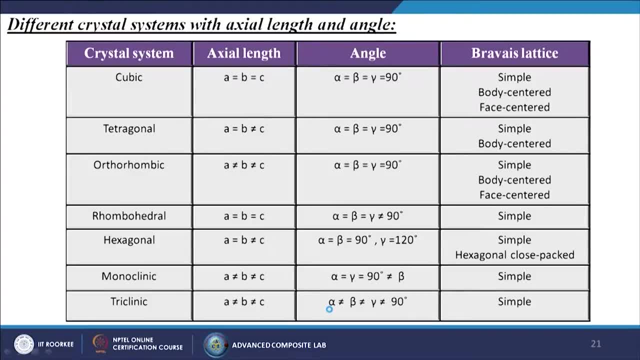 So, total, these all are the different, These all are the different types of Bravais lattices. So now we are going to discuss about the different crystal systems with axial length and the angle. So for generally cubic, as I told already, it is A, is equal to B, is equal to C because 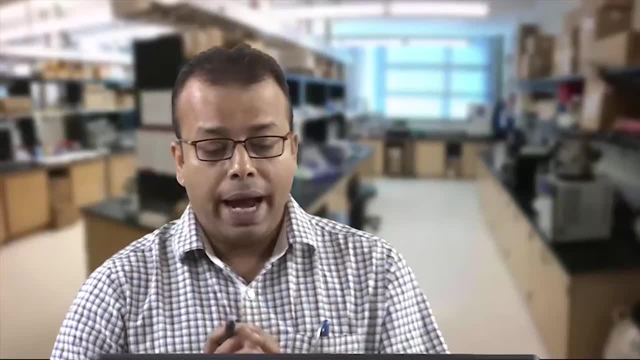 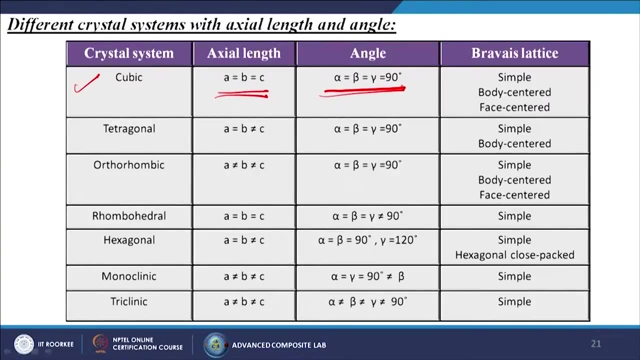 all the length are same because it is cubic angle. it is perfectly 90 degree to each other. so alpha is equal to beta, is equal to, gamma is equal to 90 degree. Bravais, lattice, it is simple. generally, sometimes it is body centered. 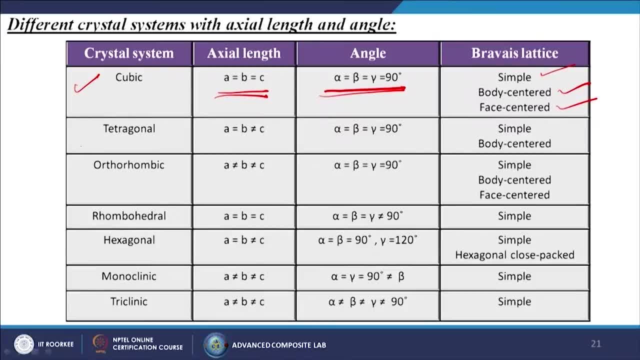 Sometimes it is face centered. also We are talking about the tetragonal. it is a is equal to b, not is equal to c. Alpha, beta, gamma is equal to 90 degree. generally it is simple and body centered, one Orthorhombic: a, not equal to b, not equal to c, is equal to alpha is equal to beta and gamma. 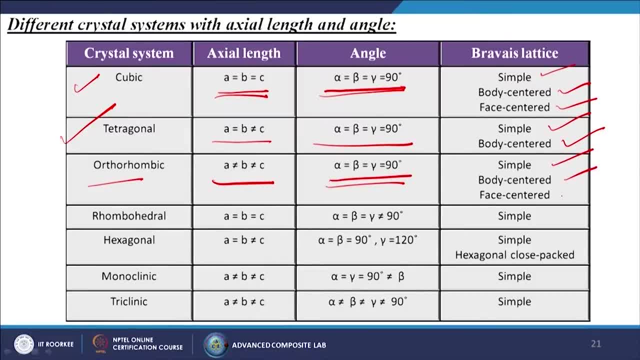 all are 90 degree. it is simple: body centered and the face centered. When we are talking about the rhombohedral, a is equal to b, is equal to c, is equal to A, is equal to B, is equal to C. alpha, beta and gamma are not 90 degree. it is simple. 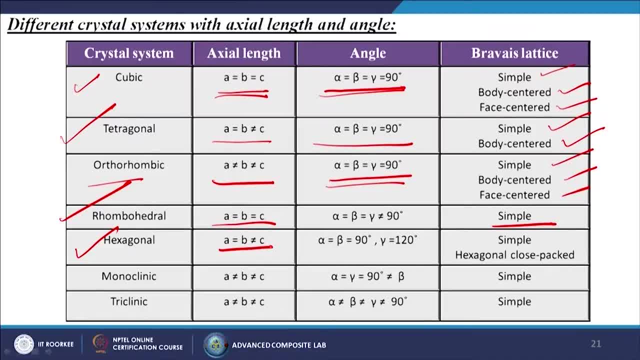 it is hexagonal: A is equal to B, but not is equal to C. alpha beta is 90 degree but gamma is 120 degree. it is simple, hexagonal, close backed, Then monoclinic: A not equal to B, not equal to C, alpha is equal to, gamma is equal to. 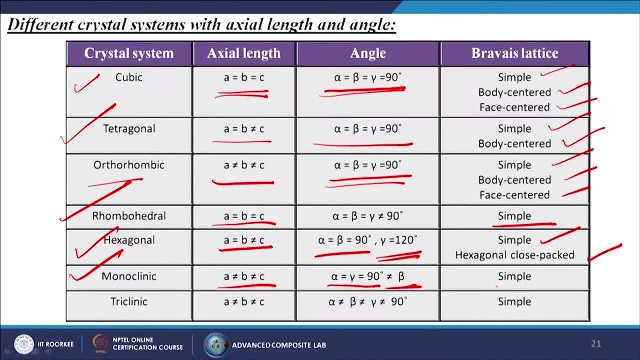 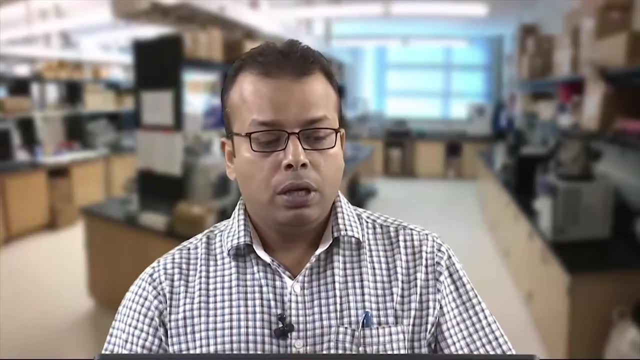 90 degree, but not the beta. it is simple. Next one is the triclinic. it is A not equal to B, not equal to C, alpha not equal to beta, not equal to gamma, not equal to 90 degree. it is very, very simple. 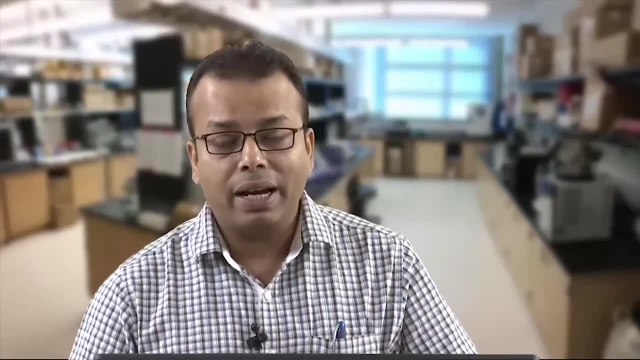 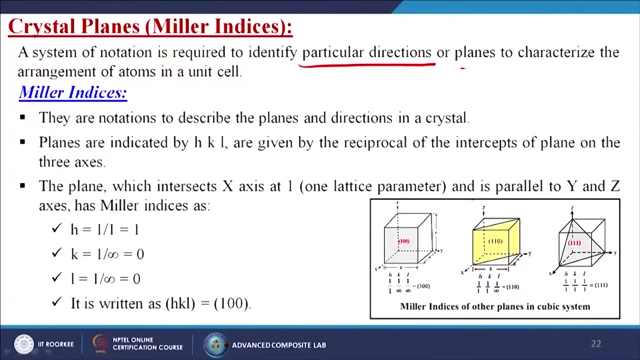 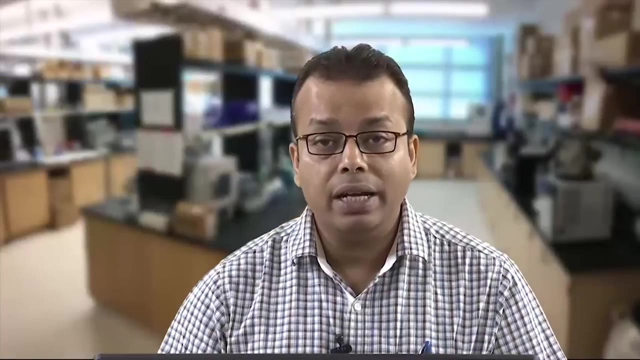 So now we are going to discuss about the crystal planes, that is, Miller indices. a system of notations is required to identify the particular directions or planes to characterize the arrangement of atoms in a unit cell. Now it is the very interesting one that is called the Miller indices. 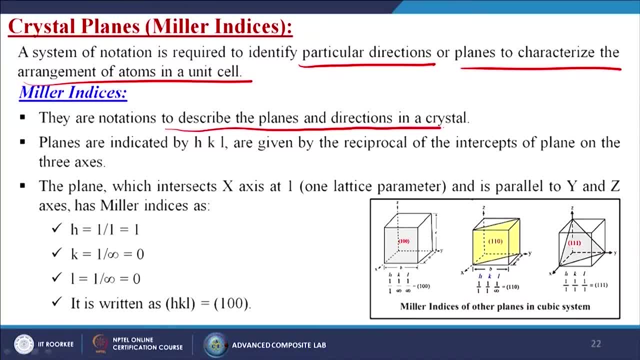 So they are the notations to describe the planes and the directions. in a crystal Planes are directed by H, K, L are given by the reciprocal of the intercepts of plane on the three axis, so 1 by H, 1 by K and 1 by L. 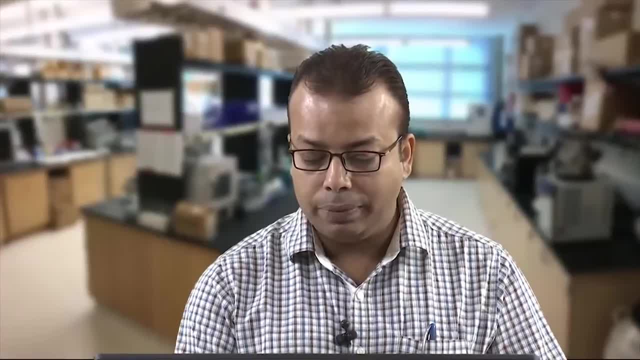 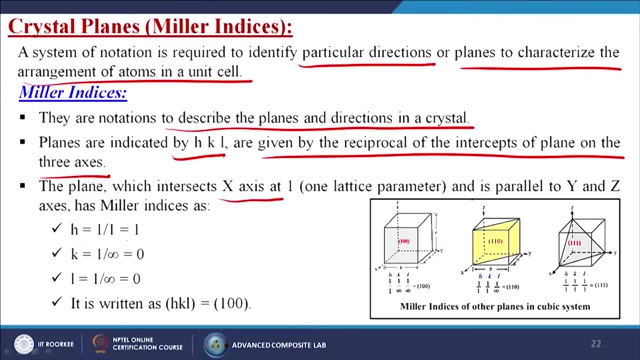 So the plane which intersects X axis at 1, 1 lattice parameter and is parallel to Y and Z axis, This has Miller indices like: H is equal to 1 by 1 is equal to 1, K- 1 by infinity, is equal. 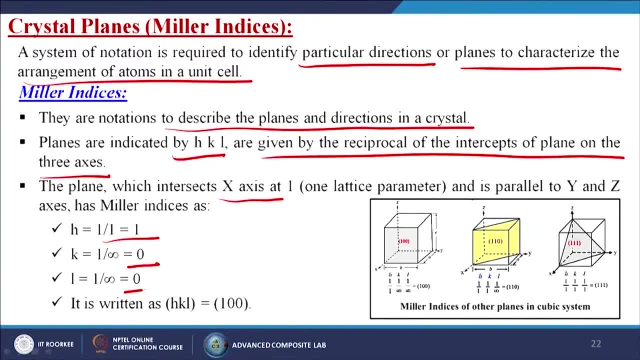 to 0 and L 1 by infinity is equal to 0. So it will be written as H K, L value 1, 0, 0. So in this particular case, so you are having, X is equal to 1, so this is your starting. 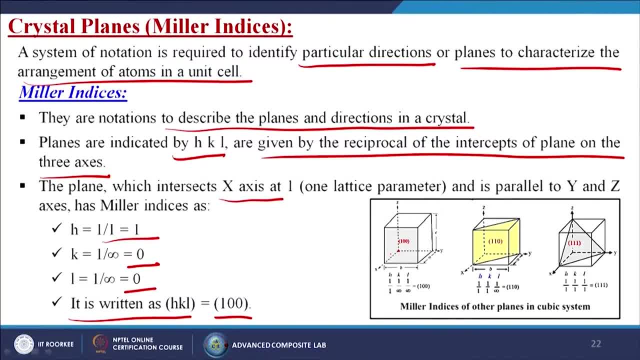 point. So from this you will come. so you will come one unit over here, and then your K and L value is almost 0, so Y and 0, so you were talking about this plane itself. So that is the plane. Then you are coming to 1, and then your L is also 1 is going, but this is 0, so you are. 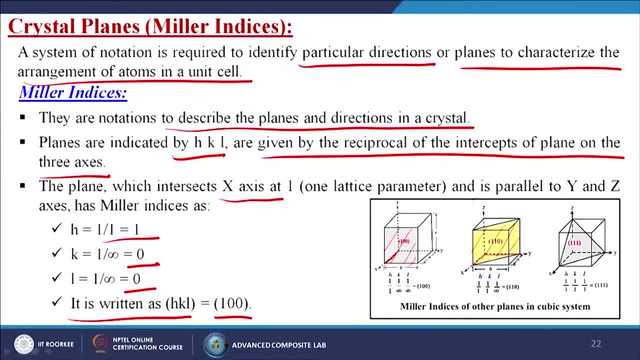 talking about this plane itself. that is plane and is this plane only. So this is known as the plane. So like, this way we can calculate the total plane of that particular crystal structure. So Miller indices directions. vector of convenient length is placed parallel to the required. 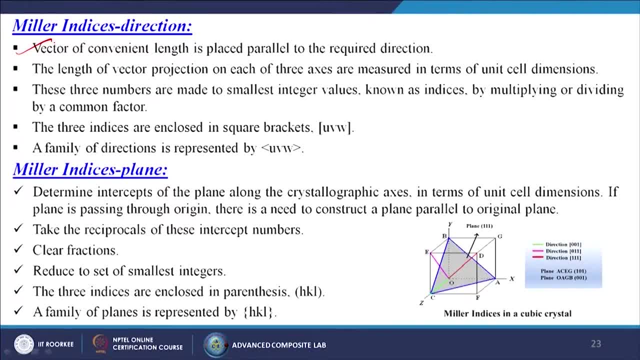 directions. the length of vector projection on each of three axis are measured in terms of the unit cell dimensions. these three numbers are made to smallest integer value, known as indices, by multiplying or dividing by a common factor. The three indices are enclosed in square brackets, like this way in the third brackets: UVW. 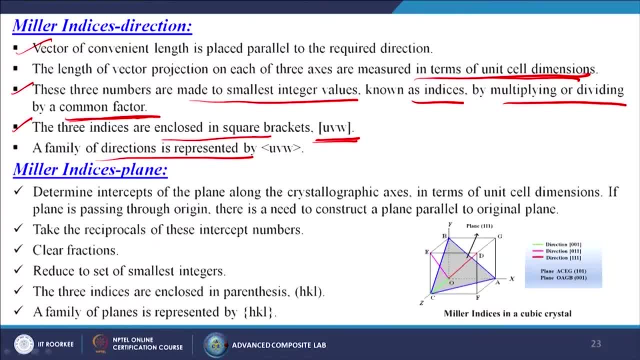 a family of directions is represented by in this manner. so less than UVW greater than Now. we are going to discuss about the Miller indices plane. so determine intercepts of the plane along the crystallographic axis in terms of unit cell dimensions, if plane 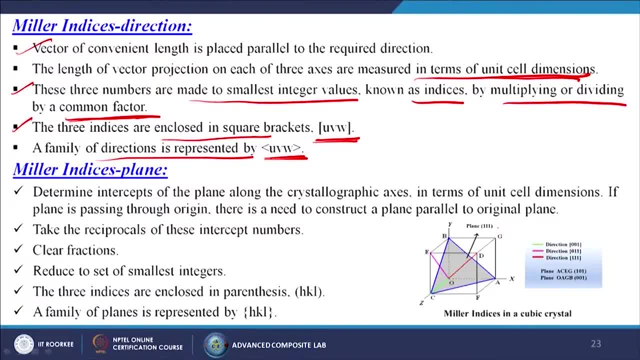 is passing through the origin, there is need to construct a plane parallel to the original plane. So take the reciprocals of this intersect numbers. so first you are making a plane, so it is passed through the origin itself. so now take the reciprocal of this intercept. 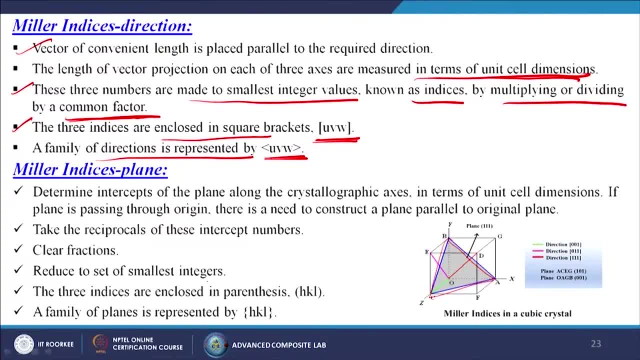 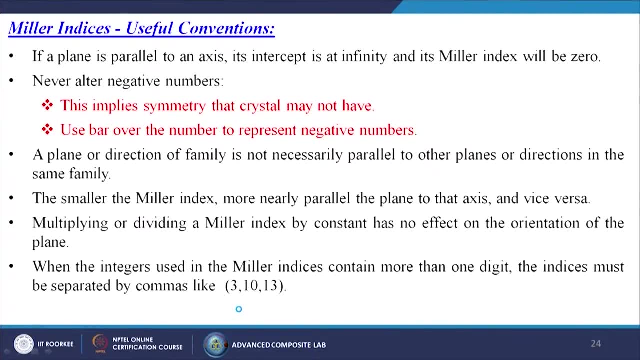 numbers. clear fractions reduce to set of smallest integers. the three indices are enclosed in parenthesis, like first. within first bracket, HKL. a family of plane is represented by second bracket, that is HKL. Miller indices: useful conventions: If a plane is parallel to an axis, its intercept is at affinity and its Miller indexes will. 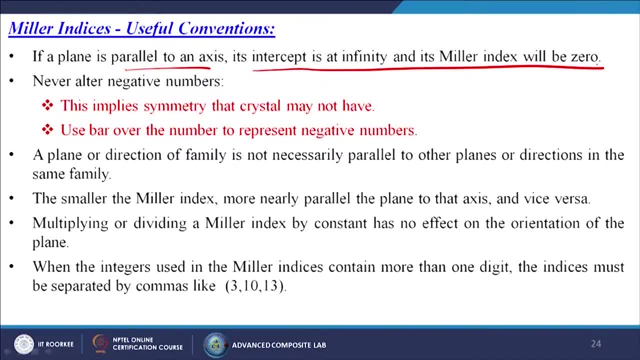 be 0, never alter the negative numbers. this implies symmetry that crystal may not have or maybe use bar over the number to represent the negative numbers if it is minus 1, so generally we are giving it as a 1 bar. So a plane or directions of family is not necessarily parallel to other planes or directions. 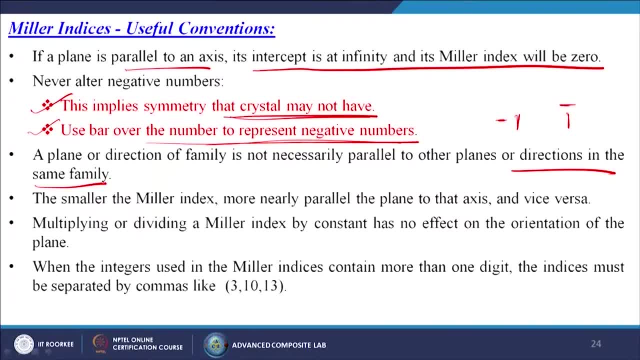 in the same family, the smaller the Miller index, more nearly parallel to the plane to that axis, and the vice versa. multiplying or dividing a Miller index by constant has no effect on the orientations of the plane itself. when the integers used in the Miller 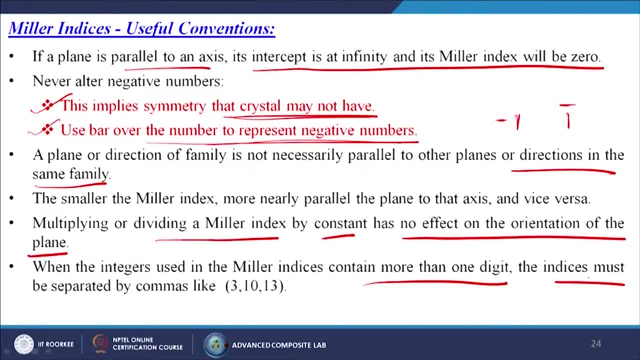 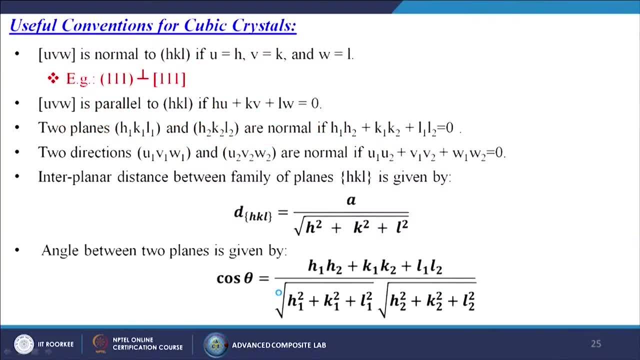 indices contains more than one digit. the indices must be separated by commas, like 3,10,13, and so on. Now some useful conventions for the cubic crystals. so U, V, W in within the third bracket is normal to HKL, is U is equal to H, V is equal to K and W is equal to L. example 1,: